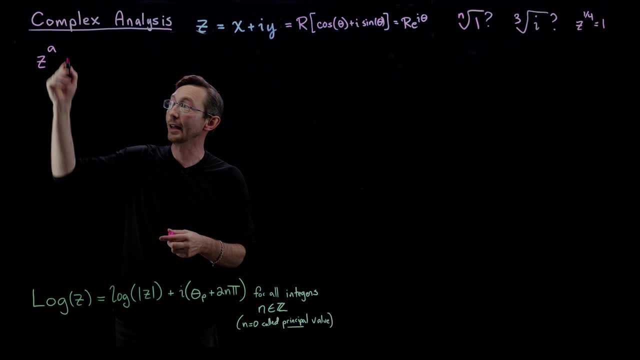 We're talking about functions: z to the power a, where a is no longer an integer. We know how to take z squared, z cubed z to the fourth power, and so on. How do I take z to the one third power? 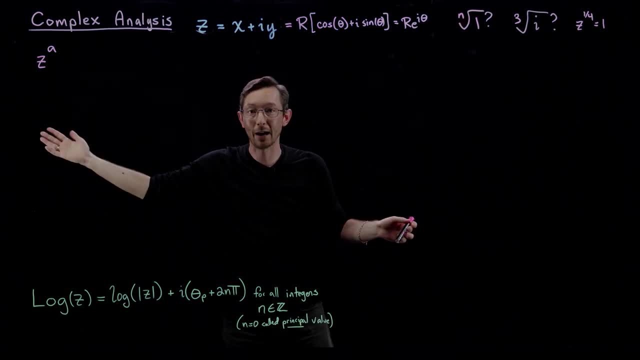 Or z to the one nth power. How do I take z to the one nth power, And so I'm going to do a little? or z to the pi-th power. How do I do things like that? And we're going to use the complex logarithm to do it. 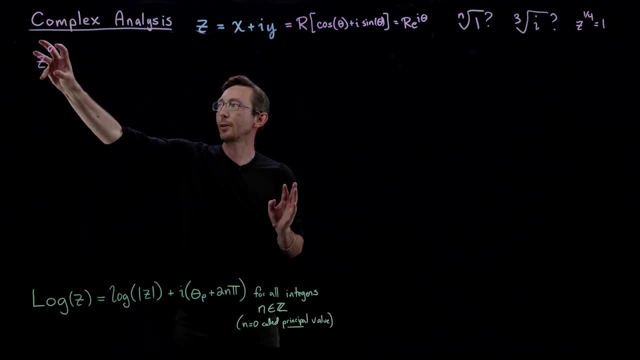 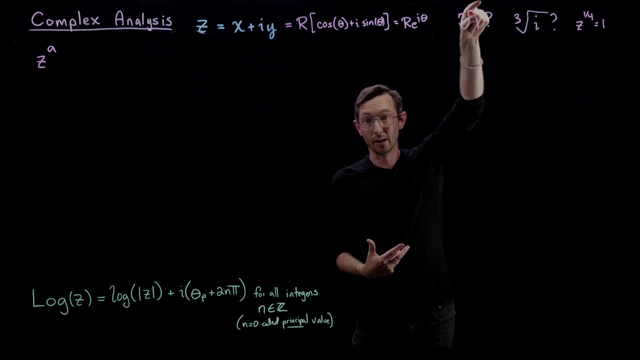 So maybe the first thing I'll do is I'll tell you how we're going to analyze these functions, because it's going to allow us to do things like compute the n roots of 1 or the 3 roots of i. We already know that the square root of a number- there are two square roots. 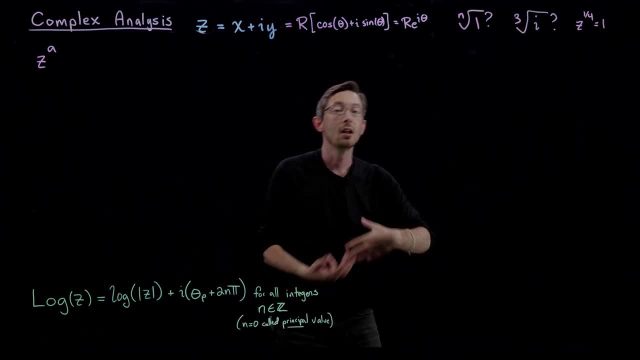 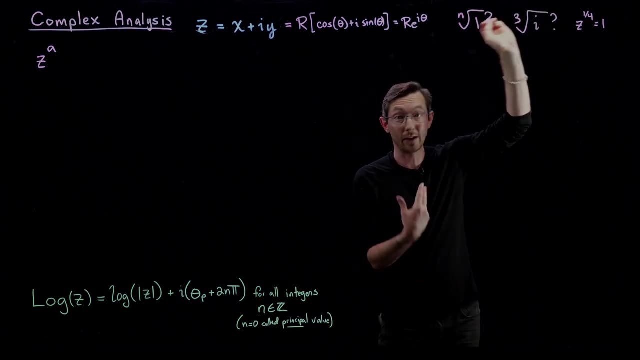 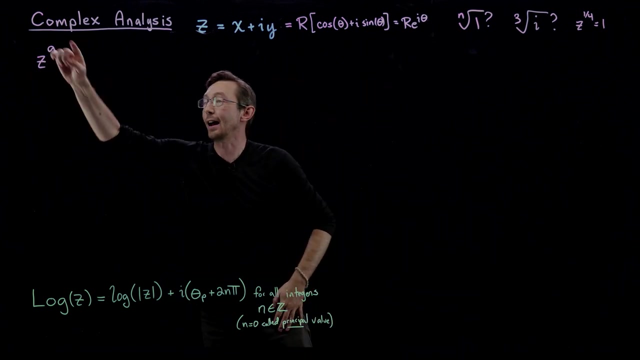 The square root of 9 could be plus 3 or minus 3.. The square root of negative 1 could be plus i or minus i. Similarly, there are three cubed roots of any complex number. There are n. n-th roots of any complex number, z, and we're going to figure out how, using this complex. 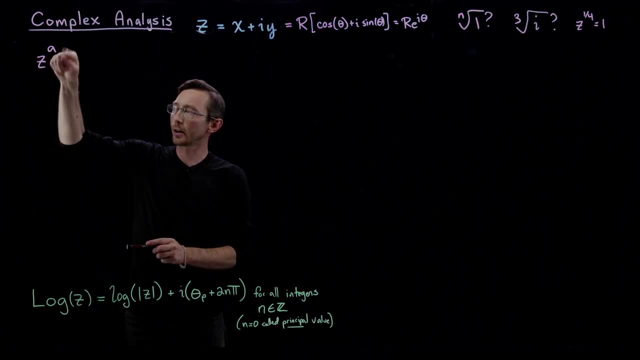 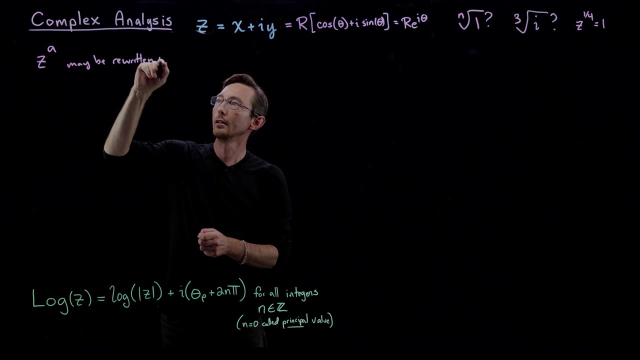 logarithm formula. So the first thing we're going to do is we're going to rewrite this z to the a using exponentials and logarithms. So we're going to rewrite. essentially, this may be rewritten, re-written using exp, the exponential function, and 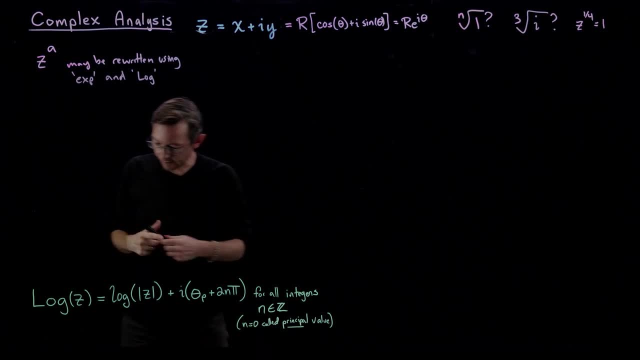 log, the logarithmic function, And specifically the way we're going to do that is we're going to say that z- Sorry, let me think. Yeah, so z is going to equal e to the log of z. Log of z is infinite valued, but e to that only has one value. That's the way I'm going to explain this again in a way. 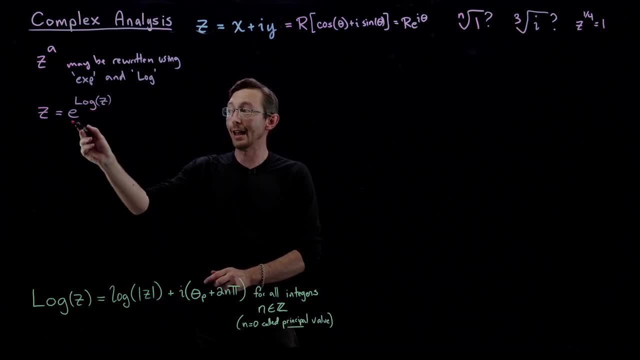 that's less confusing. So this is definitely true, because log and exponential are inverse functions. If I take the log of z, all of these values, but then I exponentiate any one of them, I recover z. So this is definitely true. 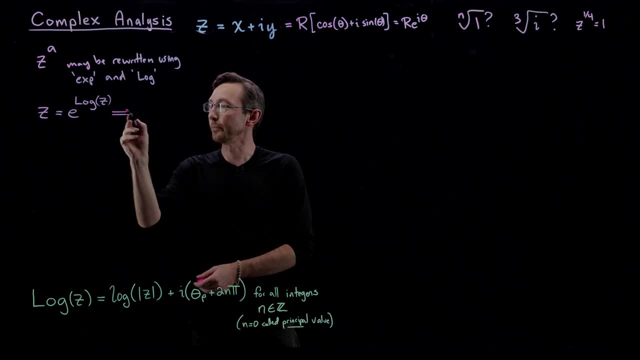 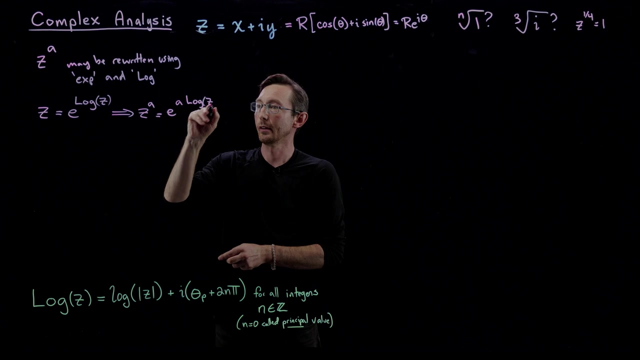 And so we're going to essentially use that to show that z to the power a is equal to e to the. it's this to the power a, which we also know is e to the a log of z. So we're going to take this expression for log of z, We're going to multiply it by that. 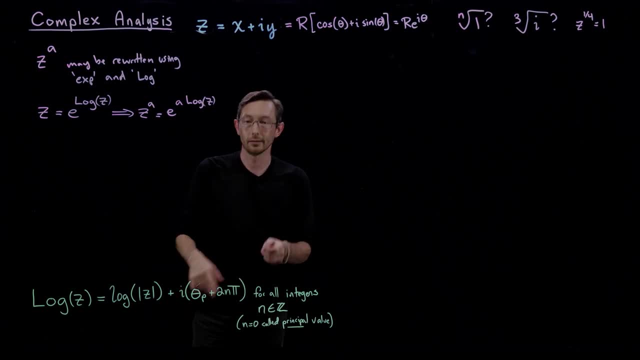 power a. so a log of this plus ia times that, And we're going to see what falls out when we take the exponential of that And that's how we're going to define, find functions like z to the 1 half or z to the 1 third or z to the negative 1 third, things like 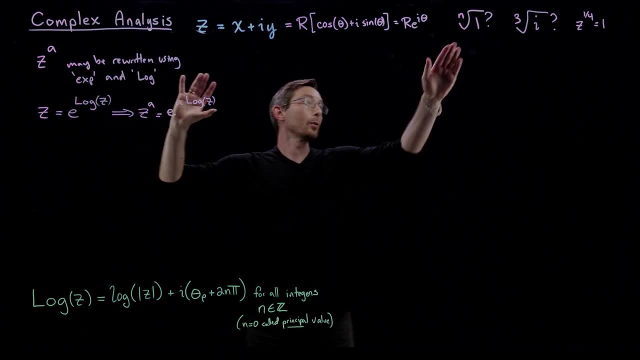 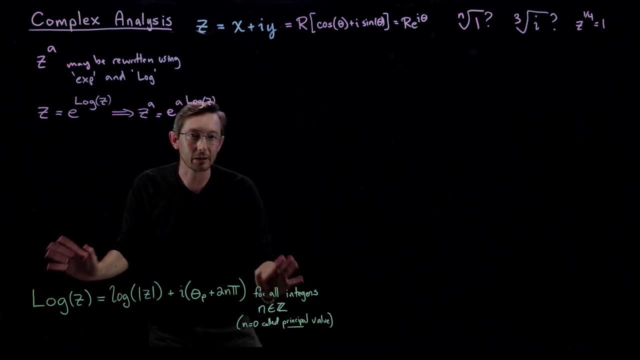 that okay. Now, before we get into this and before we solve, for you know, the square root of i or the third root of i or things like that, I'm just going to very, very, very quickly recap why this logarithm was infinitely valued and why that's not actually that confusing at all, okay, So? 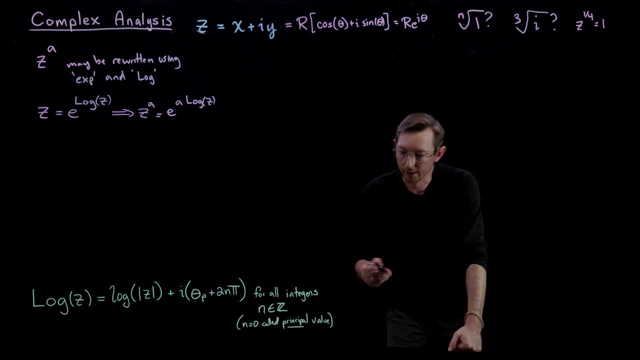 specifically we wanted. if we think about z in the complex plane, so z is this number in the complex plane and it has a radius and it has a principal angle between 0 and 2 pi, just the way we always define angles between 0 and 2 pi. If I add another 2 pi to that theta, it's exactly the. 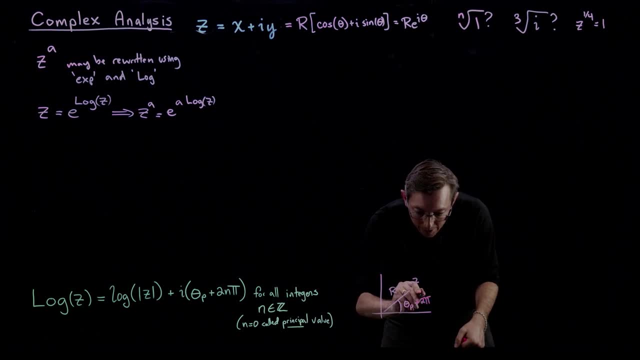 same point. So plus 2 pi n is exactly the same point as long as n is an integer. So when we say n is an element of the integers- this is just a math way of saying n is an integer- then this z could be defined using: 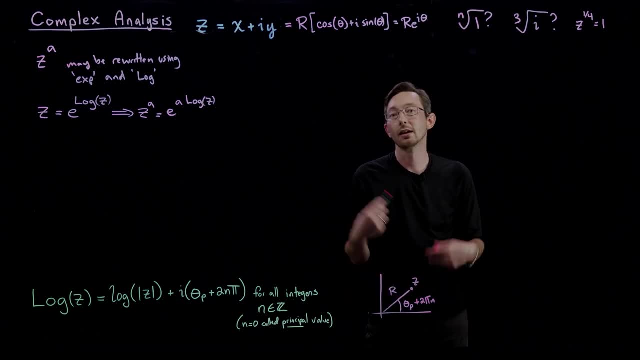 any of those angles. Let's say, this was, you know 30 degrees. 30 degrees is fine, so is 390 degrees. So you know, if this was you know pi sixths, then pi sixths plus 2 pi is also. 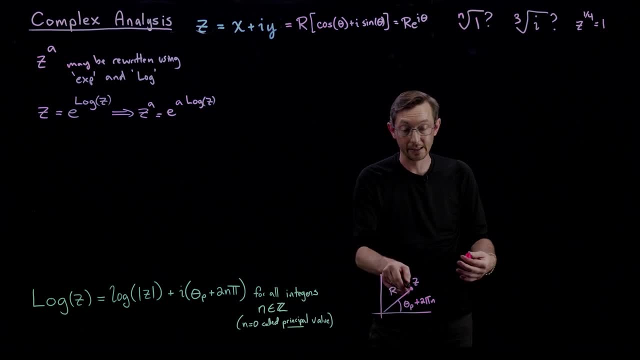 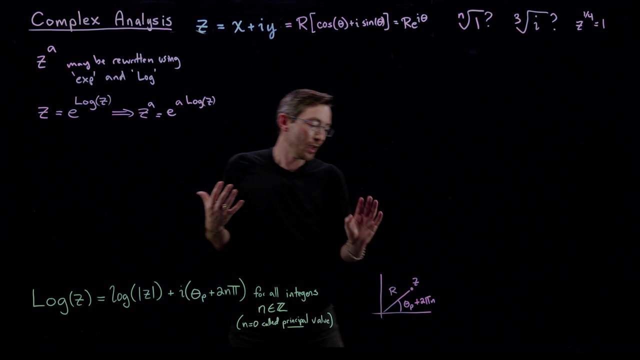 valid Plus 4 pi is also a valid way of defining z. We normally only choose the principal value between 0 and 2 pi, but I could add 2 pi to that any way I like. And the real catch here- I think what was confusing last time for me, I confused myself- is that if I add 2 pi n to that, 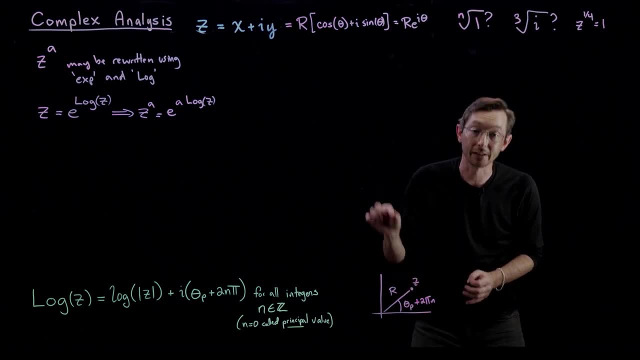 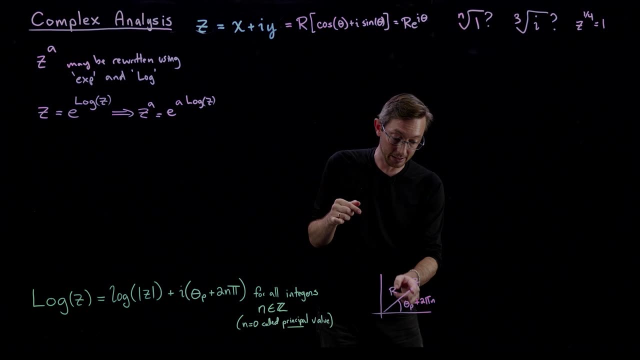 phase angle this value z doesn't change. It's not like there's infinitely many. you know z's z is x plus iy. There is a single real value x and a single real value y. that uniquely defines that complex variable z. But in the phase angle way of writing it, there are infinitely many. 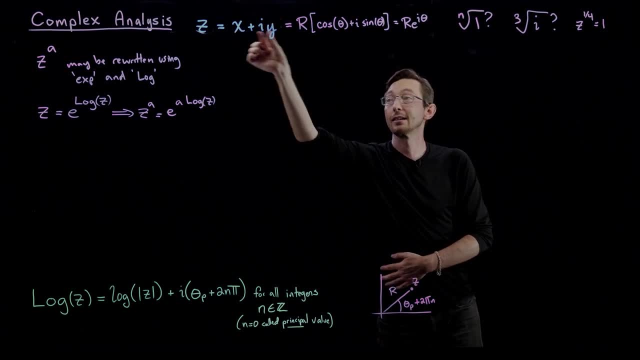 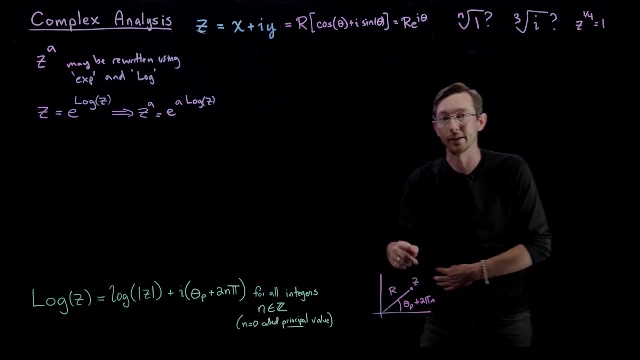 thetas that are equally valid for getting that real x and that real y. I could use the principal theta, theta pi, or I could add 2 pi, add 4 pi, add 6 pi, Just because there's different ways of. 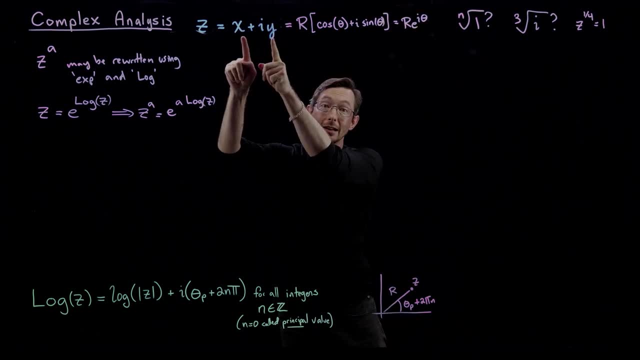 writing it in the complex plane. it doesn't mean that it's the same thing. So if I add 2 pi doesn't mean there are infinitely many z's. There's just z. It's a complex number. It's a. 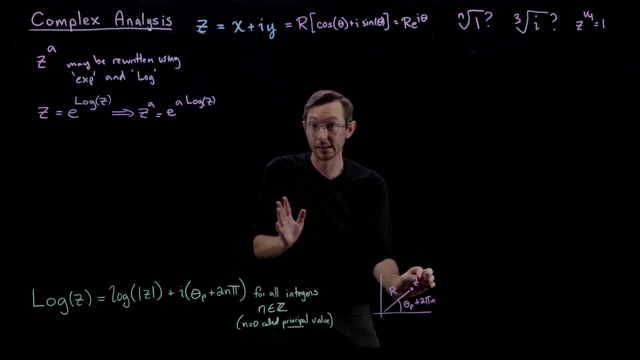 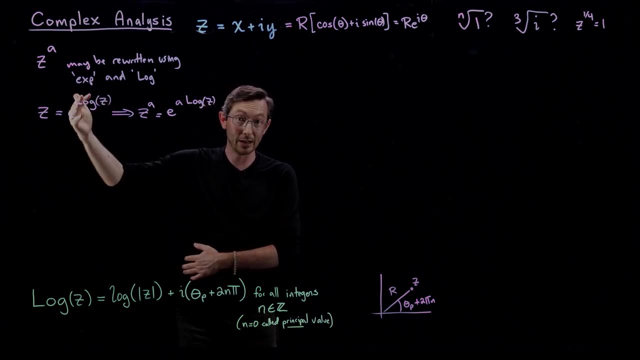 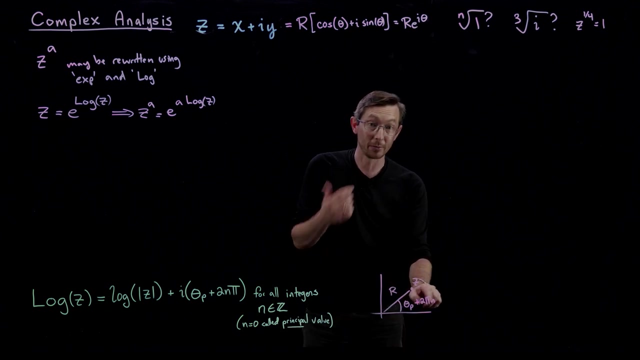 real thing that exists and it has. you know, there's one value, z, But when I compute the logarithm, specifically so that the logarithm is the inverse of the exponential function, now all of those many, many ways of writing that phase angle in terms of adding multiples of 2 pi. 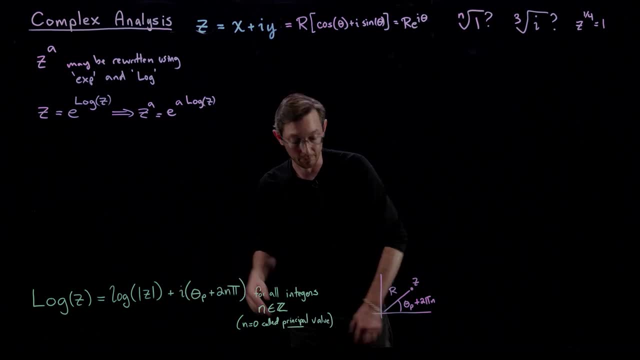 are all valid for this complex logarithm, Because the logarithm of z is specifically log of the magnitude of z. sometimes we call this the radius. this is just. you know, r plus i times any angle. that if I took e to this angle, 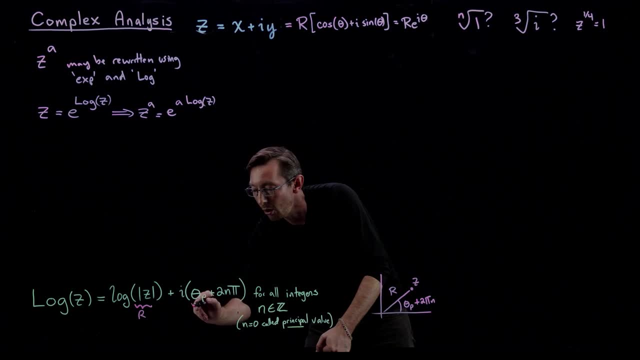 you know it would recover z. And now, all of these infinitely many angles are all valid, Because if I took e to this number for any integer n, I would recover z Now, even though there was only one z in the first place. there really are infinitely many. 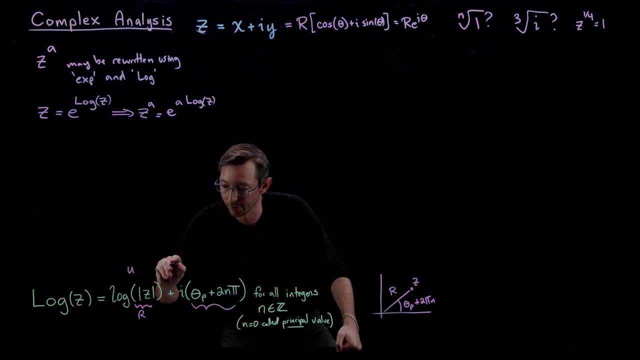 log of z's. This is, you know, u plus i v, And these actually are different v's. It's not like here where, just going around, I get to the same place, the same exact z value Here if I add 2. 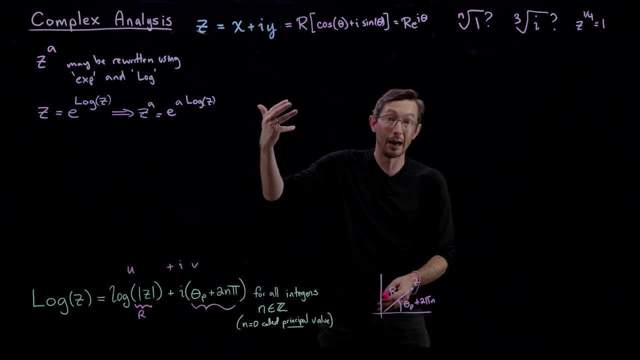 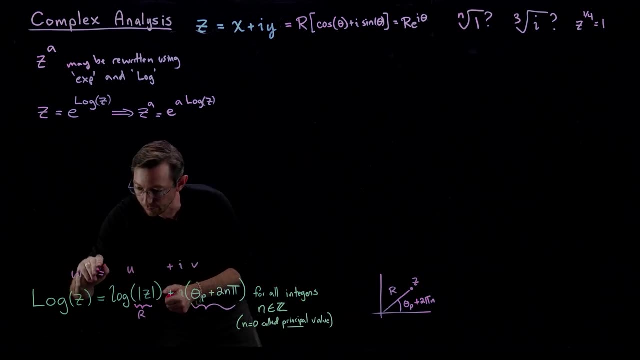 n pi. I have a new v. v is actually 2 pi n bigger, You know. so there's this number. v equals. actually changes when I rotate around, you know, and I add 2 pi to this phase angle of z. 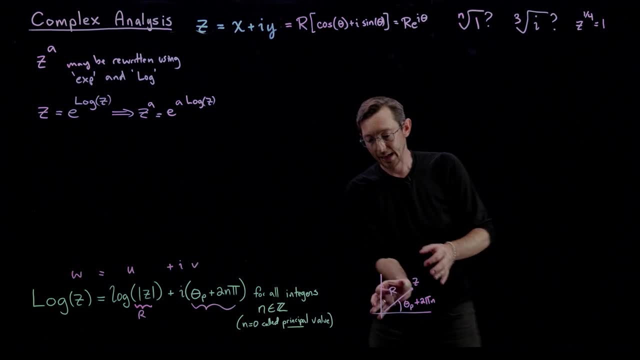 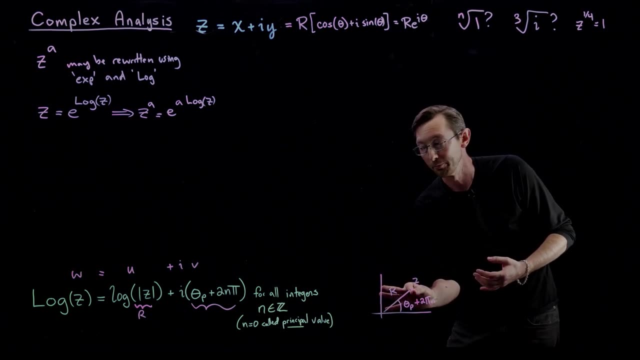 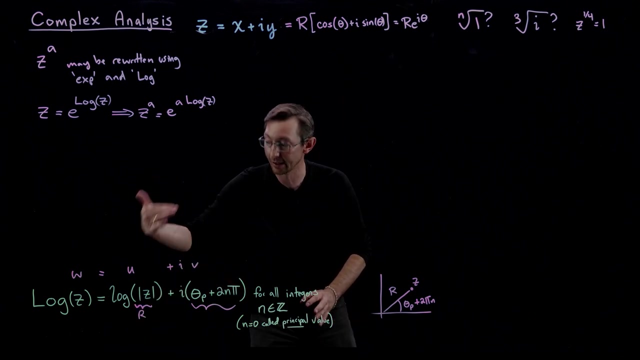 So I think that's where it gets really interesting to me is that this input variable z, is uniquely defined. It has one value. This is one value, But the logarithm- there are many, many values for this v- that when I took e to that u plus i v, I would recover z. 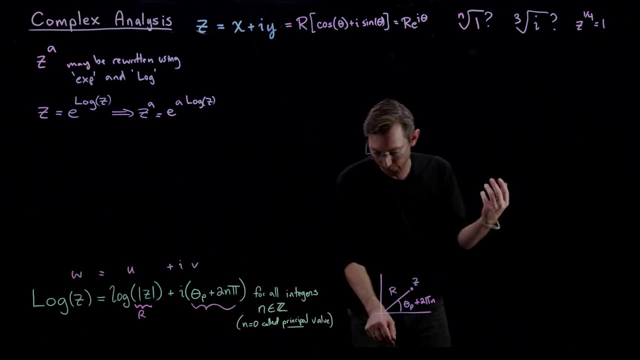 And these are actually different values. v in that complex logarithm. The way we drew it before was, you know, this is the z plane. The w's that are valid are all on this line, real w equals log of the radius. But then I have many, many values for this v term, for this phase angle. 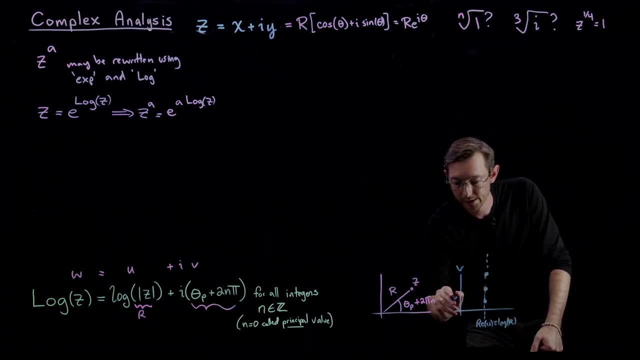 here that are all valid. So there's the principal theta, And then plus 2 pi, plus 4 pi, you know plus 6 pi, 8 pi, 10 pi, minus 2 pi, and so on and so forth. 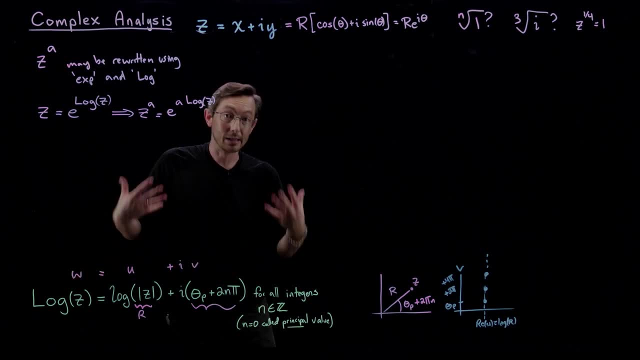 So I just wanted to clear up. It's not that weird that this complex logarithm is multi-valued. It's a property of the fact that there are many ways of writing this phase angle. I could add 2 pi i as many times as I like to this phase angle, and this value of z doesn't change. 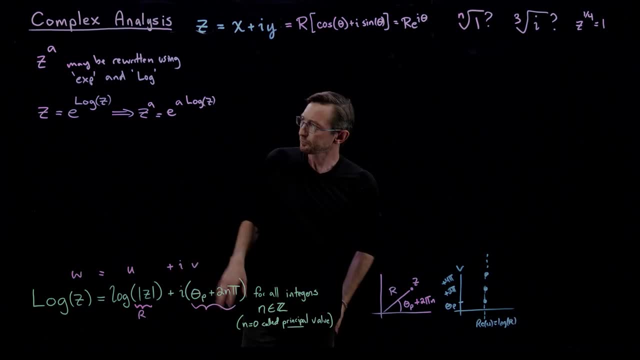 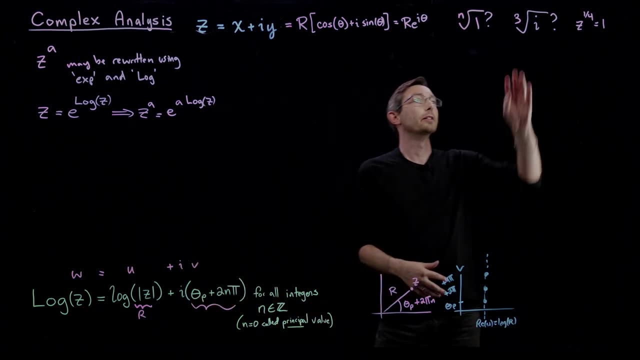 But those are all valid logarithms of z. Good, So we're going to use that property, that this is infinite value, that this is true for any integer n to define. you know what is the cubed root of z? What is the square root of z? the fourth: 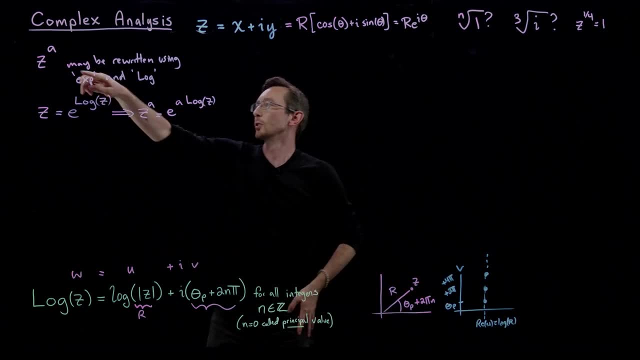 root and so on and so forth, the nth root of z. So we're going to, you know, for example, example this could be. you know, for example, eg, for example, z to the 1 half is the square. 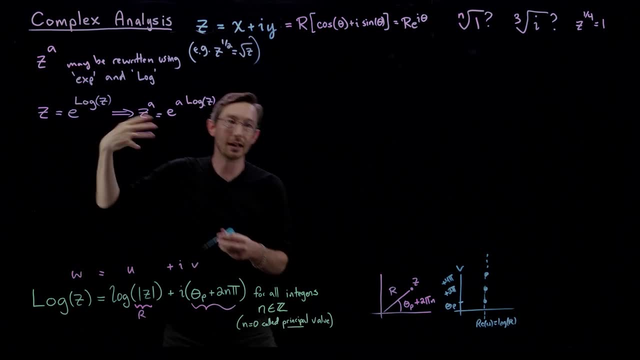 root of z. So you know, if a was 1, half, I'd be computing the square root of z, things like that. So I want to define what these functions are. We know what z to an integer is. What is z to a fraction like one, half or two? 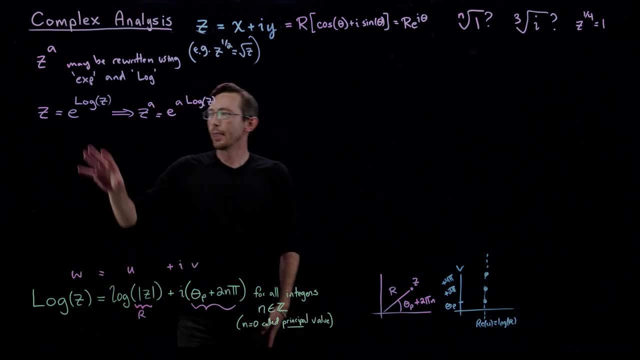 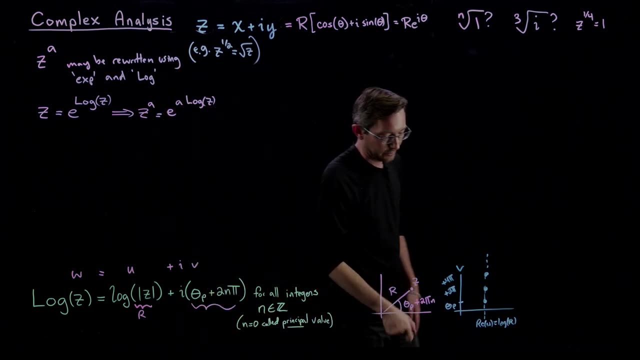 thirds or something like that. Okay, good, And this is the basic formula we're going to use to define that quantity. Now, before I actually take this logarithm and plug it into this formula, I want to give you an example. I want to give you an example of what is the cubed root of one. 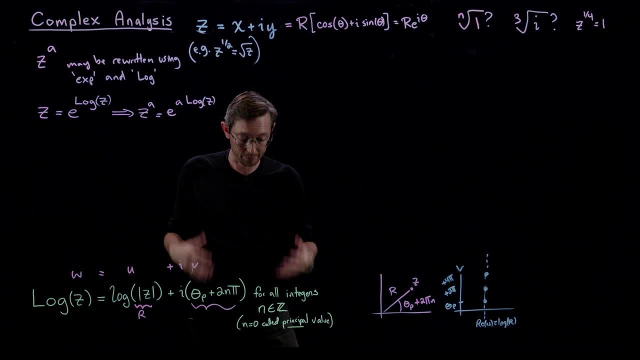 okay, Because I think this is something that everybody's going to understand and it's a pretty simple concept. So I'm going to draw my. how do I want to do this? I'm going to draw my complex plane and I'm going to draw the. so here's the problem we're going to solve. 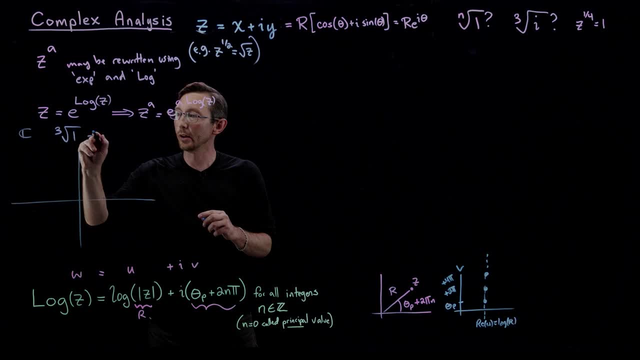 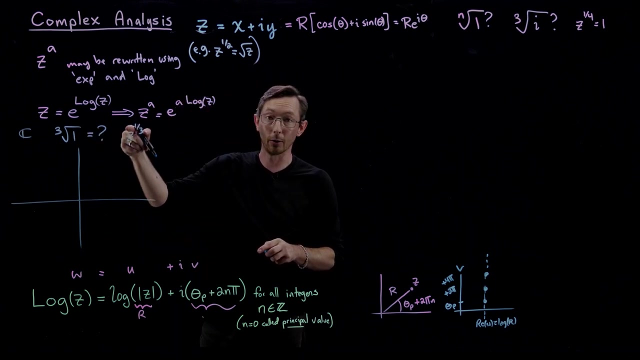 We're going to say: cubed root of one equals what? Okay, so that's another way of saying. you know, z to the one third is our function and z equals one. So we're trying to understand the function z to the one third power. 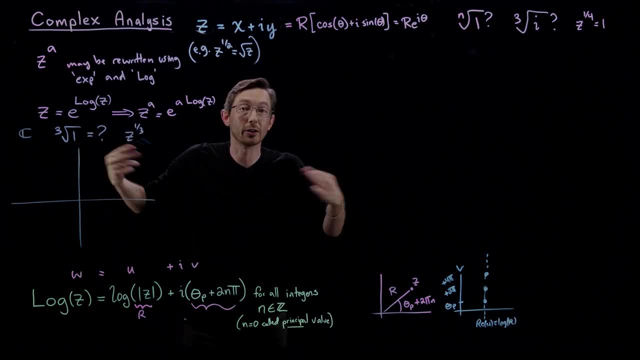 and we're evaluating that at z equals one. What are the values that are valid for z to the one third? Now we kind of know already that one of the cubed roots of one is one, because one to the cubed, you know, to the one third, is one. So we're going to draw our function and we're going to 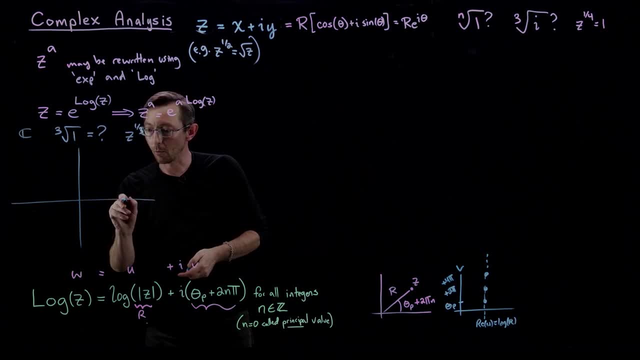 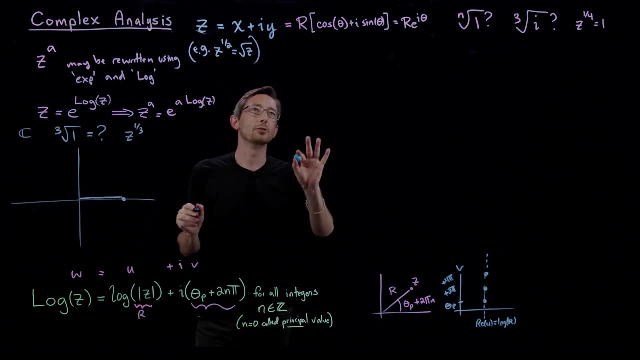 to the third. power is one. So I know that one of the cubed roots of one is going to equal one And I'm going to call that e to the zero. We know that one equals e to the zero. That's just saying. 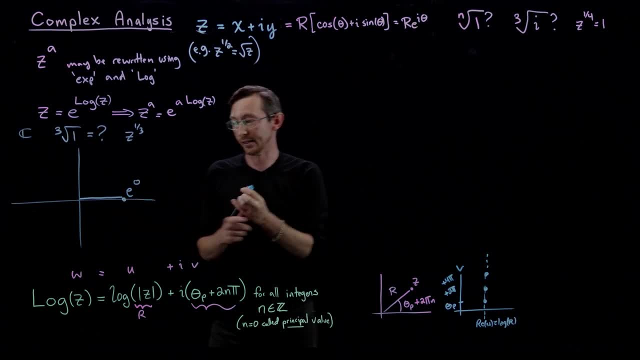 radius equals one, theta equals zero. This is e to the whatever, i zero, if you like, e to the zero. But what's interesting is that, if I took- how do I want to write this? Let's say that this number the cubed root of one. let's call that, you know, let's call that. 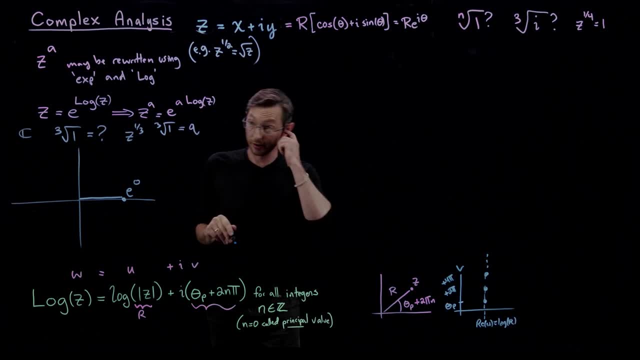 q just to be cute. So we're saying q cubed equals one, And so I know that e to the zero is one solution, e to the i zero, But I'm going to claim that two pi n. I can add two pi n to that. 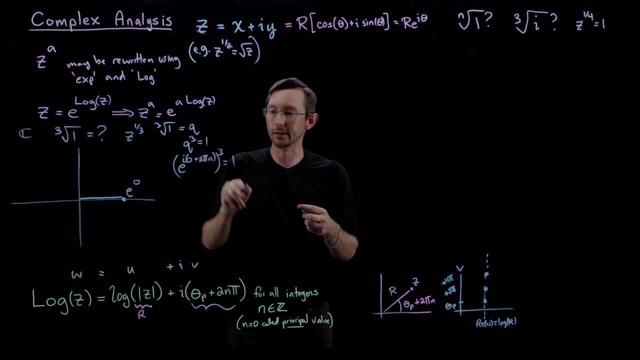 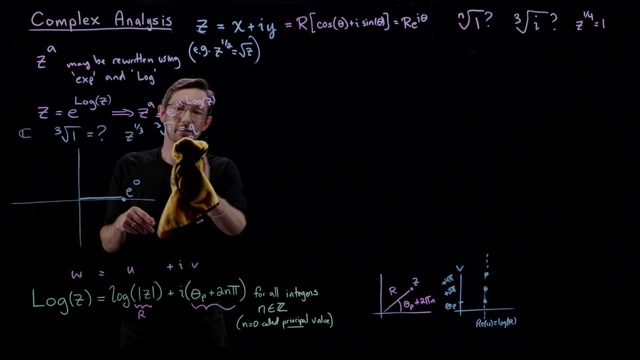 and that's also going to equal one when I cube it. So let me show you. I'm going to draw the picture, then we're going to derive this. I think this will make it easier to understand. So if I I'm just going to draw the answer because I think I want to show you, 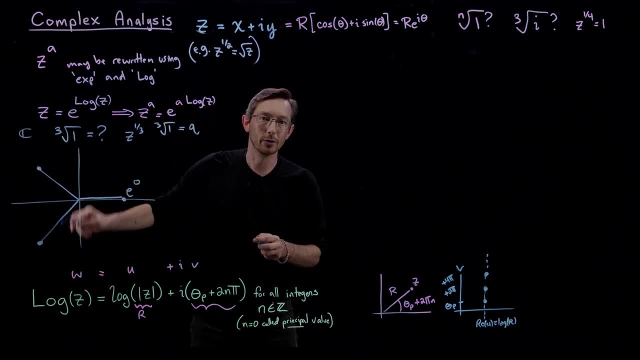 and then explain: These are the other two cubed roots of one. There are three numbers that if I cube them I will get one, which means specifically this angle here, this theta, So so so this e to the zero, this is the principal cubed root of one. 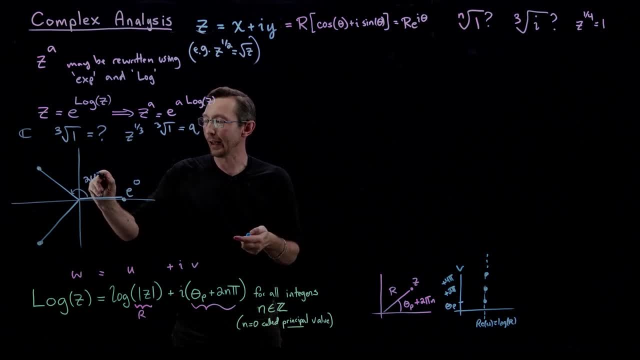 But if I take, you know, two pi divided by three and add that to the phase angle, that's another cubed root of one. So if I take, you know, two pi divided by three, that's another cubed root of one. Still radius one, but now my, this is the phase angle, If I 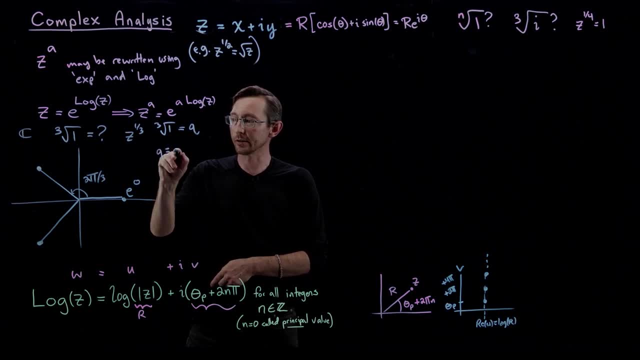 take. if I take a number, you know, q equals e to the i two pi thirds, and I cube it. cubed is e to the i two pi thirds times three is two pi. And what's e to the i two pi? Well, 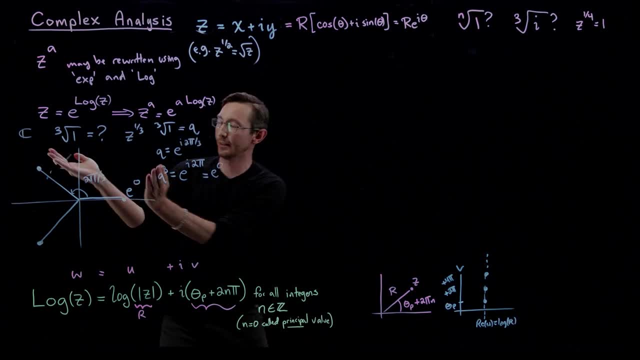 it's e to the zero. I got back to where I started. So if I take this wedge times three, I get back to where I started. This is also a cubed root of one, And then similarly this one here which is four pi. 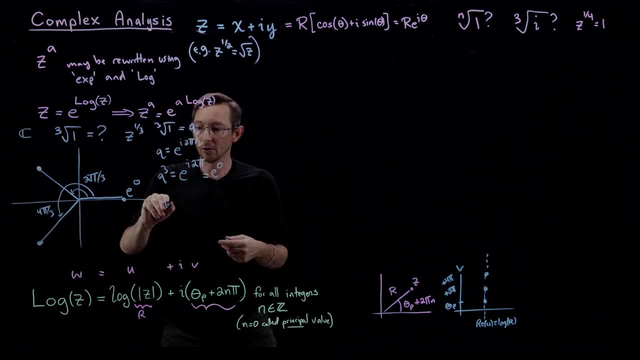 thirds is also a cubed root, Q, let's call this. you know, this is the second one. The third one is e to the i four pi thirds Again, if I take this number and I take it to the third power. 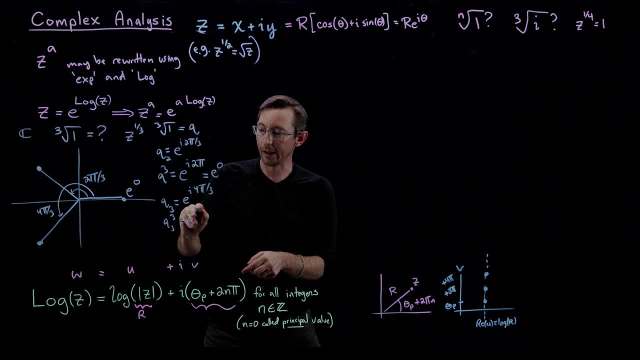 q three cubed, I get e to the i four pi. which, again, what is e to the i four pi? It's e to the zero, because if I go around two pi twice I'm right back where I started, And so you can kind of imagine if I take this. 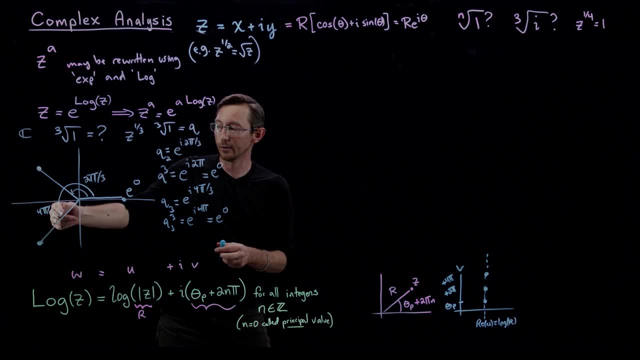 angle four pi thirds and I- this is, you know, this is q. q squared would get me here and q cubed will get me back to a phase angle of zero. So these are all totally valid cubed roots of one. I can have e to the zero. 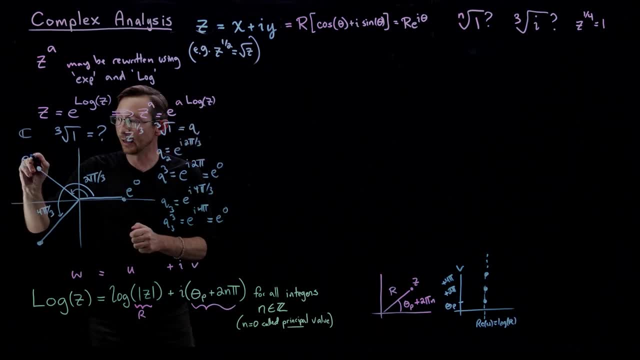 e to the. let's write this very, very explicitly: e to the: i two pi thirds. That's this point. This is e to the: i four pi thirds. Now you might think: well, why isn't there a fourth cubed root of one? Why can't I do this again? And the reason I can't do it again. 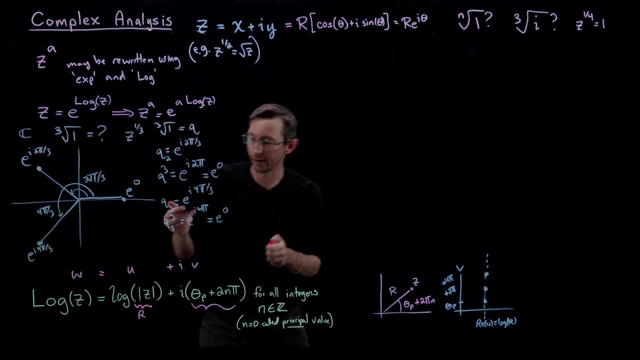 is because I'll write it in red, because it's an invalid solution. If I said q equals e to the i, let's try to do six pi, Six pi, thirds. Well, what is e to the i? six pi thirds, That's just e to the i, two pi. 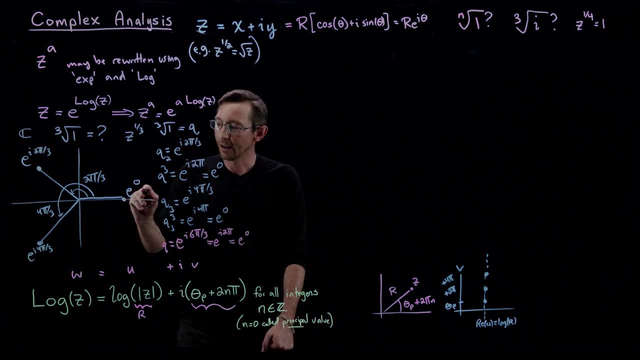 which is e to the zero. So e to the zero is e to the i six pi thirds. And so once I go around again and I can't, I can't do eight pi, because this is again. this is also e to the i eight pi. 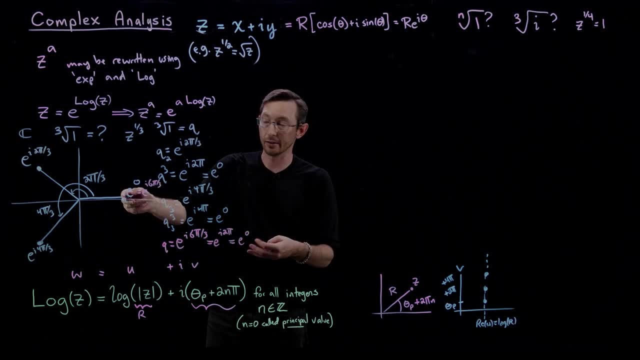 thirds, and this is: e to the i, 10 pi thirds, e to the i, 12 pi thirds, e to the i, 14 pi thirds, pi-thirds, 18 pi-thirds, and so on and so forth. So, even though I can keep adding two pi over and 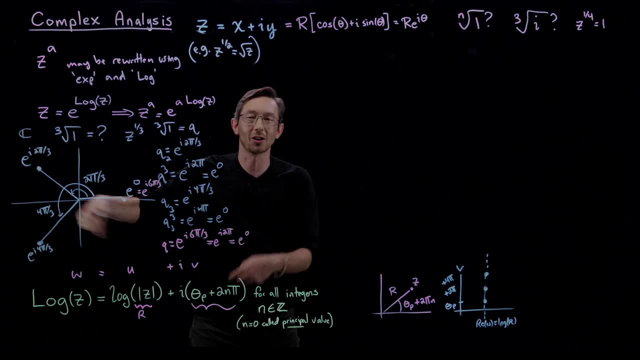 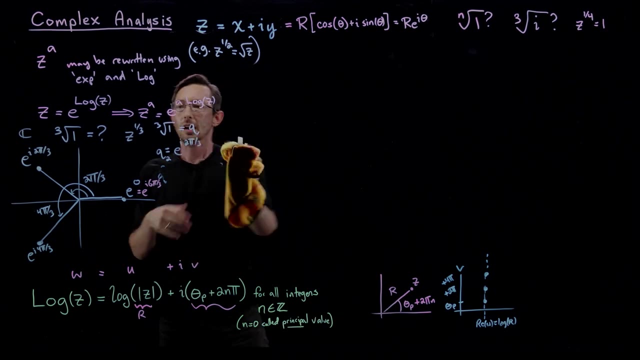 over and over, eventually those cubed roots start to be the same thing. They all mean the same thing. There's only three unique cubed roots of one Okay, so I'm going to derive the general formula and then we're going to revisit this again. So this is actually really fun and I think kind of 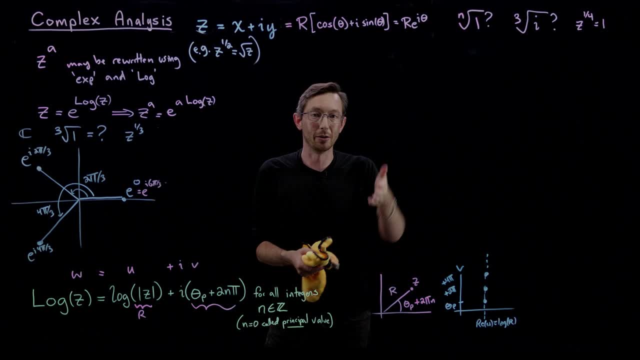 illustrative to start just playing around, Just like: pick some complex number, you know i, and compute all of its fourth roots. Pick a complex number, you know one plus i, and compute all of its ninth roots or its fourth roots or whatever. It's very, very helpful to understand what's. 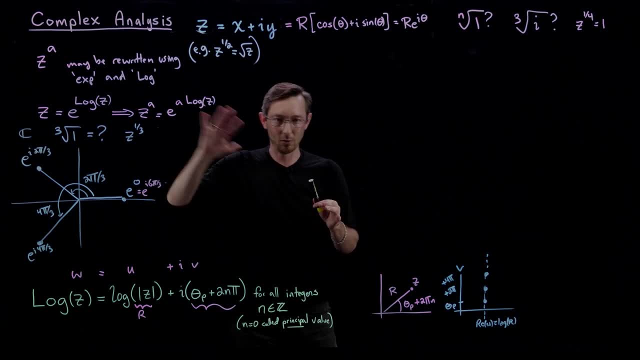 happening here. Okay, so I want to- just- we're going to revisit this- but the basic idea is that the cubed root of one- there are three values, because there are three unique phase angles- that if I cube them I'll get all the way to the bottom. So I'm going to do that. So I'm going to do that. 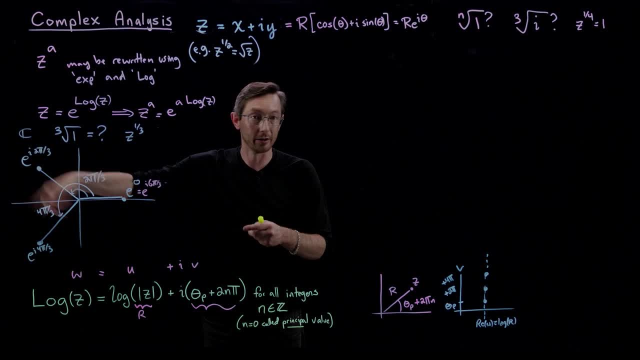 all the way back to e to the zero, or, you know, e to the 2 pi or e to the 4 pi, And there are only three unique values. because if I keep doing that trick, I basically reinvent these three solutions that I've already discovered. There's only three unique solutions. Why don't we do the same thing? 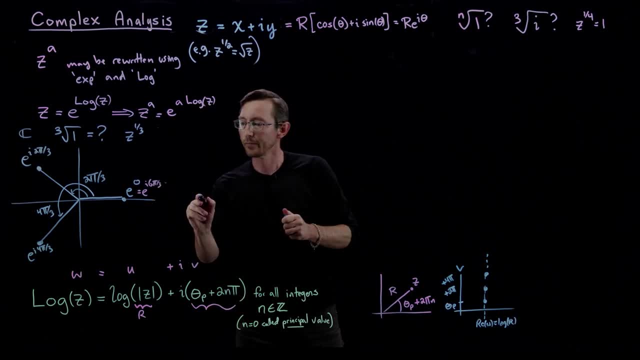 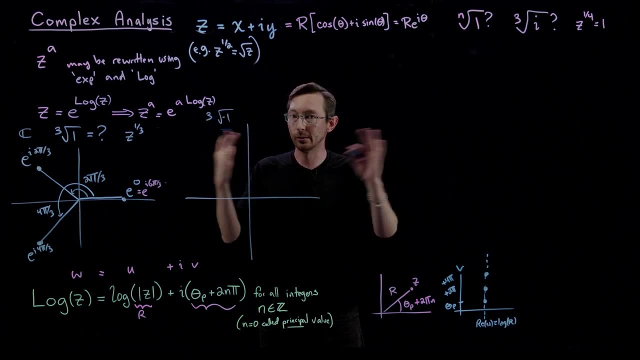 for negative one. Let's just do this again, just to make sure we understand. So let's try. you know what is the cubed root of negative one. We should be able to do the cubed root of negative one, the cubed root of i. 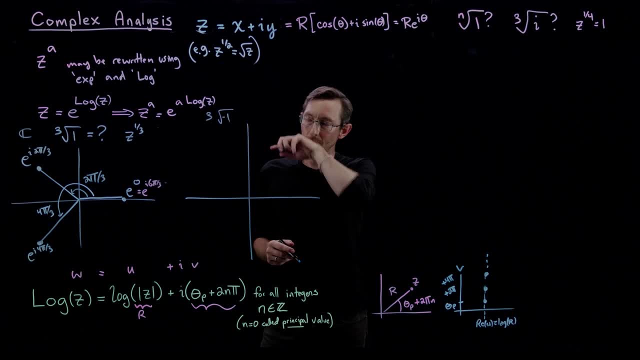 Anything we want. So again, okay, negative one is one of the principal cubed roots of negative one, because negative one times negative, one times negative one equals negative one. So this is already one of the cubed roots And this is e to the. i pi right, I've gone pi to get here. 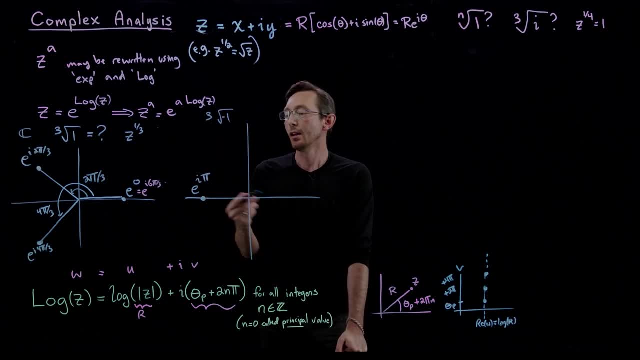 And this is what we call the principal cubed root of negative one. And again, what I'm going to do is I'm going to take 2 pi thirds and I'm going to add 2 pi thirds to this. So 2 pi thirds gets me. 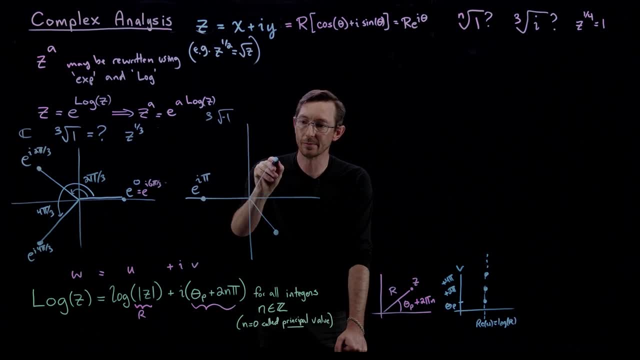 here And I'm going to add 4 pi thirds, which gets me here. And if I added 6 pi thirds, I'd rediscover this point again If I added 8 pi thirds, 10 pi thirds, 12 pi thirds. So there's. 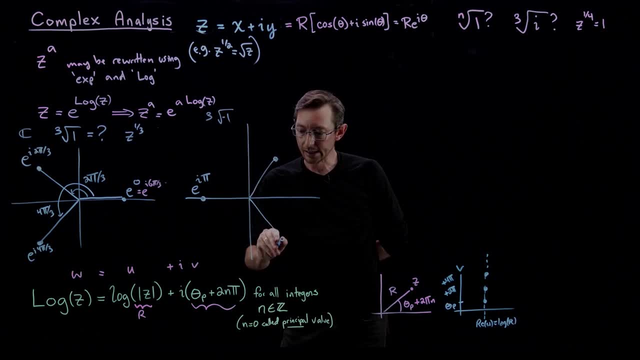 only three unique versions of this. This is e to the i pi plus 2 pi thirds. This is e to the i pi plus 4 pi thirds. And again, this is, you know, also equal to e to the i pi plus 6 pi thirds. 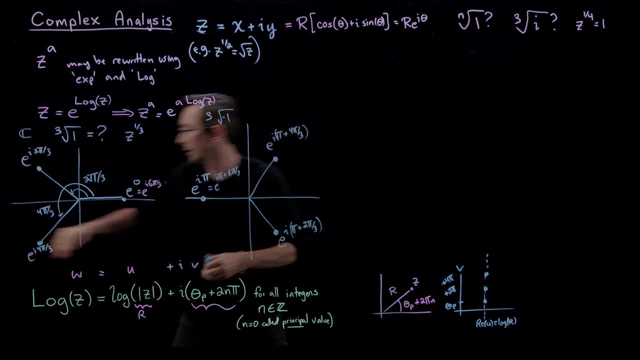 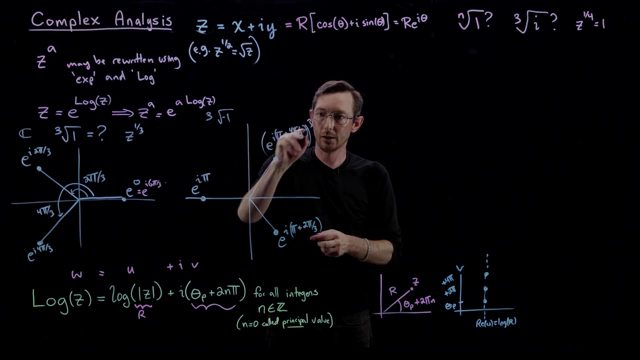 and so on. So these are kind of it repeats at some point And these are the unique cubed roots of negative one. You can easily verify that if I took this number and I cube it right, let's just take this number cubed. This cubed equals e to the i pi plus 2 pi thirds And again this is 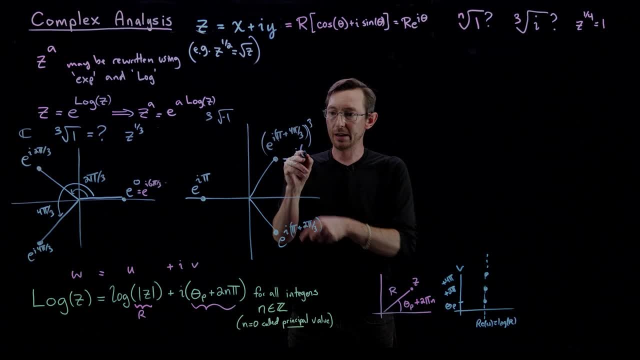 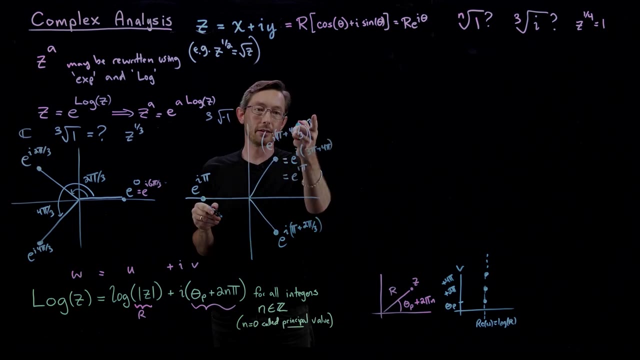 e to the i 3 pi plus 4 pi, which is equal to e to the i 7 pi. But if I go around, you know, 7 pi times it's the same as just going around e to the i pi. So this to the third power gets me. 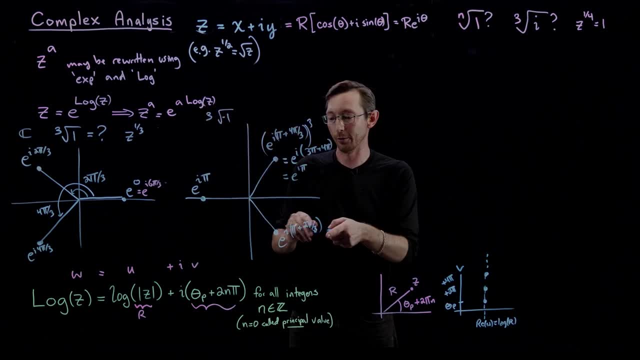 where I want to go, Similarly this to the third power, you know it'll go around, I think. instead of 7, it'll be 3 plus 8 is 11.. It'll go around, you know, and get me to e, to the i pi, So this: 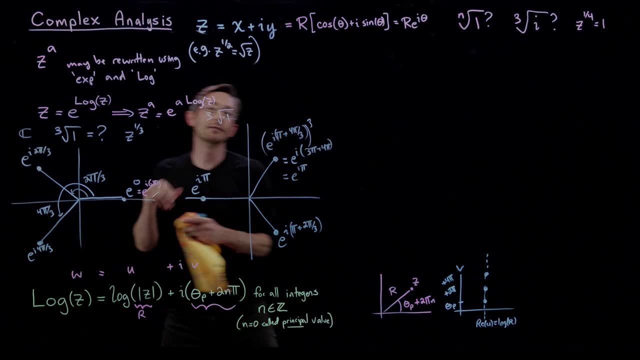 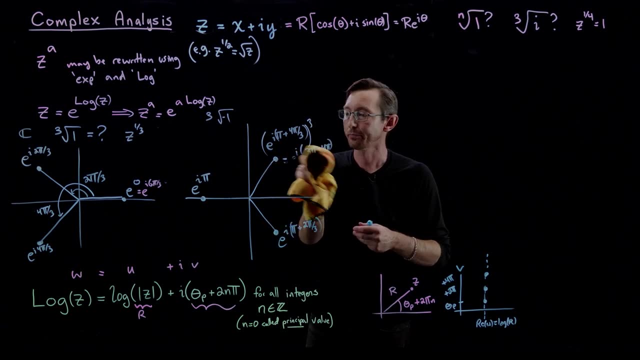 to the i pi. So these are the principal cubed roots. It's really easy to verify. Once you've found one of these, it's really easy to verify. You just take the cube of that and see if it's the number you want. Okay, good. So now I'm going to derive a generic formula for this. 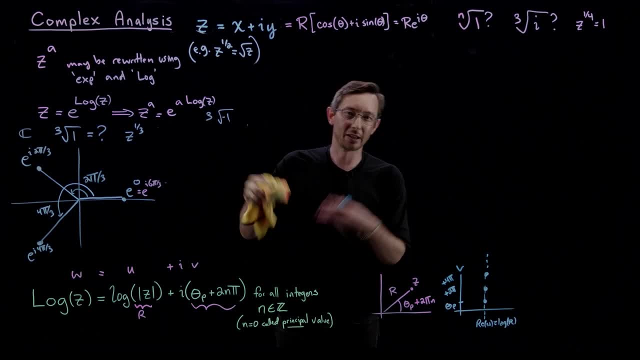 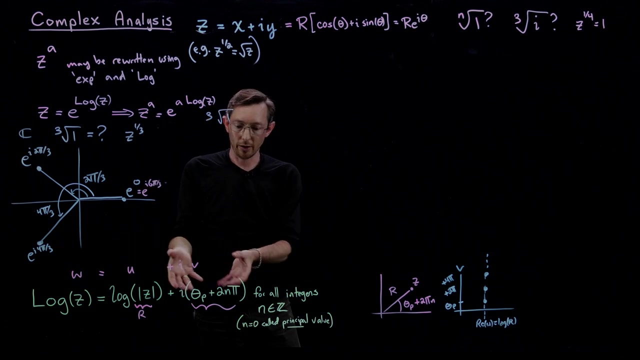 which is- and then maybe I'll do you know- the cube root of i, just because it's really useful to see one of those cases as well. So the idea here is we're going to use this expression and then we're going to show that out of all of these, 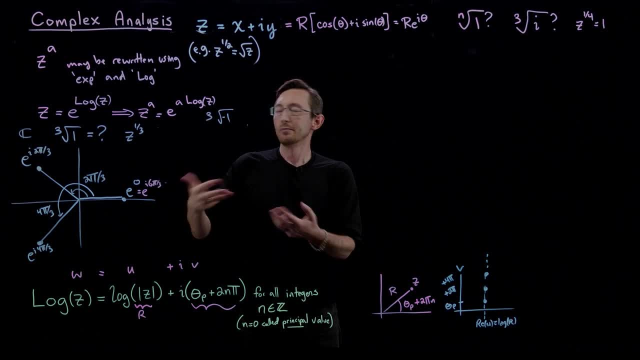 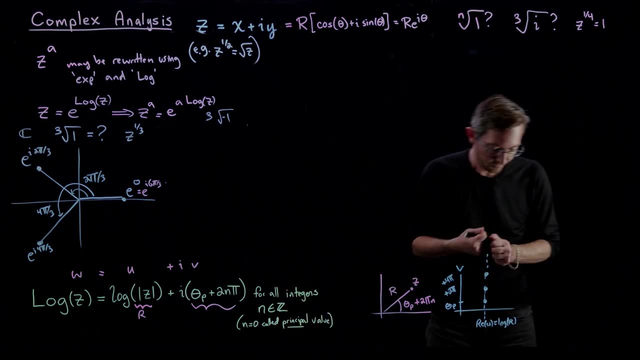 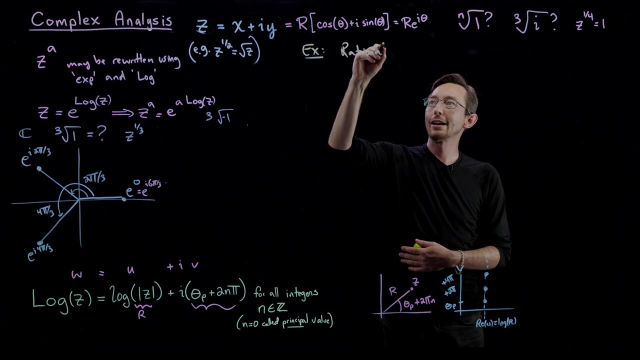 infinitely many values of log. only some of them are unique. when I'm taking z to the power a, Okay, maybe I'll use yellow here. So let's, as kind of a general example, let's take a rational a, and by a rational a I literally mean it's the ratio of two integers. So this equals: 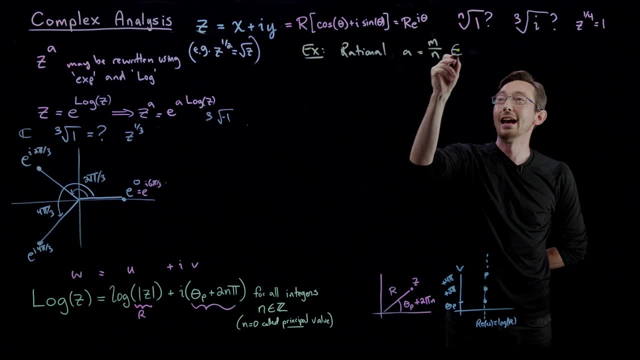 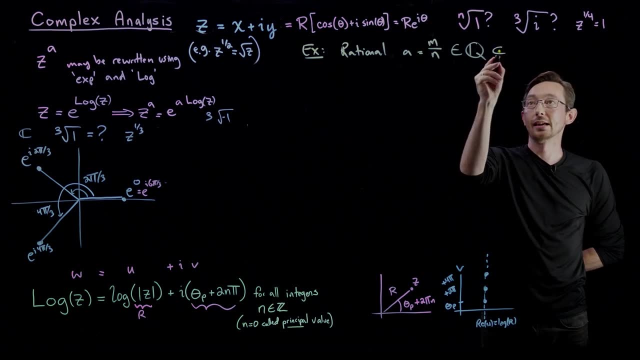 m over n. We say that this is an element of the set of rationals. That's just what in the set of rationals means, which is a subset of real numbers like pi and e and three and negative two, And what we mean is that m and n are both integers. So this is the ratio of two integers. 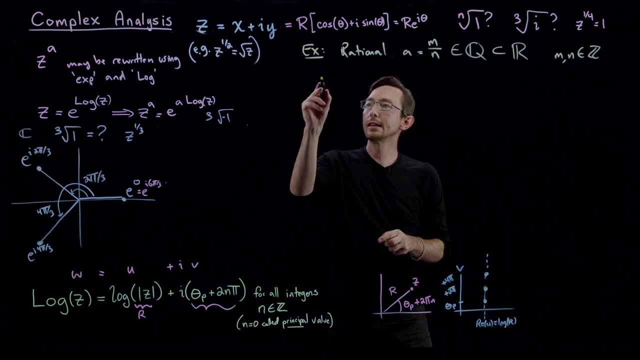 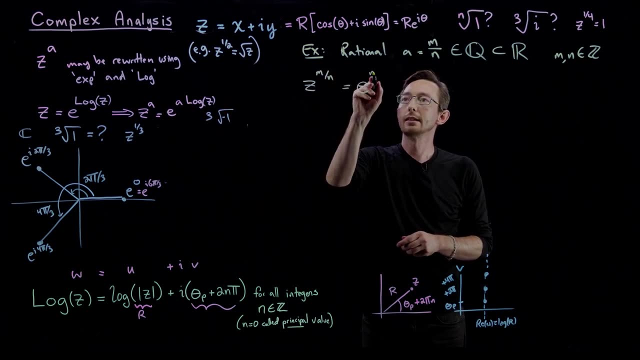 This is just the mathy way of saying it. Then what we're going to say is that z to the power m over n equals e to the m over n log of z, And I'm going to use this whole expression here and plug it in. 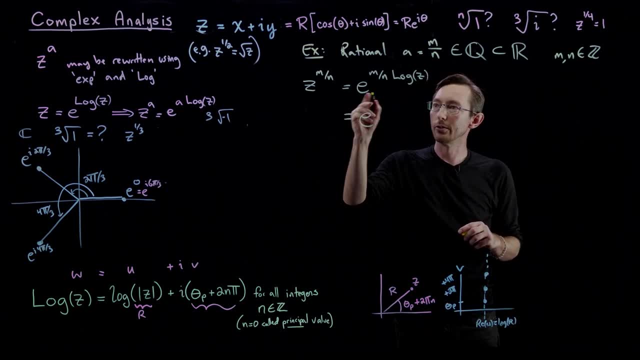 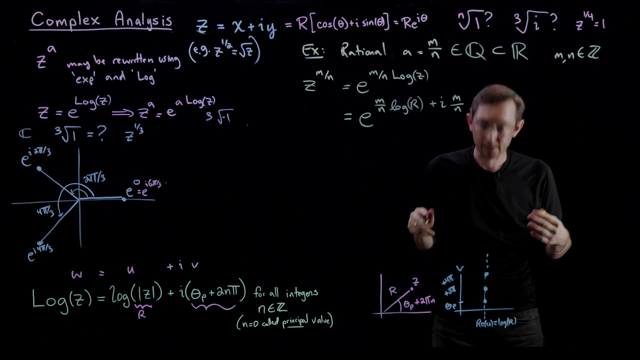 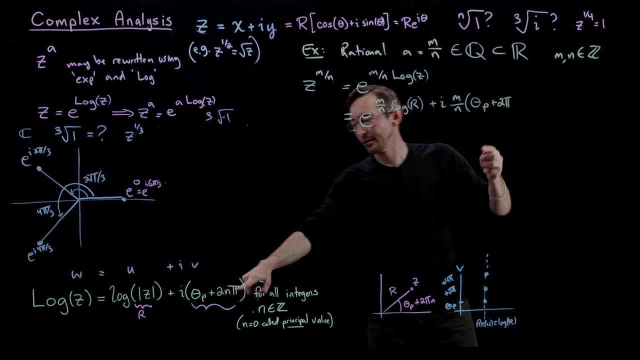 And so that's going to mean I have e to the m over n log of radius, plus i m over n times my theta principle, plus any two pi. Sorry, this is a different n here. Let's just we'll use k times, any integer times, two pi right. So this is just m over n times, the logarithm. 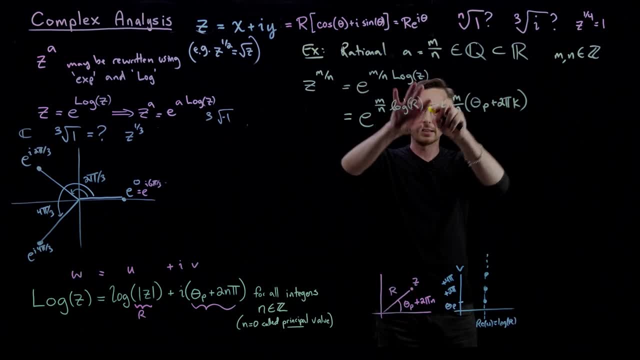 of z, okay, And I'm going to break this up into the real part, the magnitude part and the, you know, cosine and sine part. And so this equals e to the m over n log of z, to the m over n log of r. This is only one value. There's only one value here. So 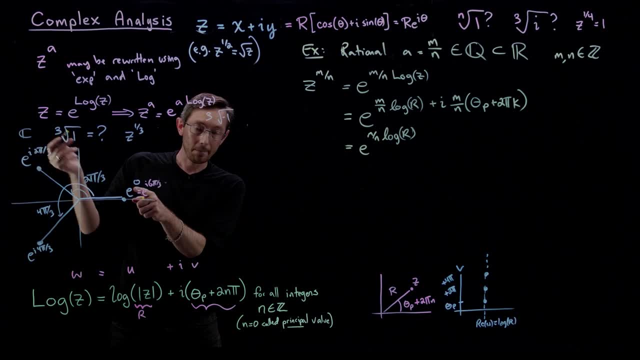 I was taking the third root of one. If I took the third root of eight, then the I would have to take the third, then the radius of that would be the third root of eight. okay, So if I took the third root of eight, that would be- you know the magnitude of that- would be the third root. 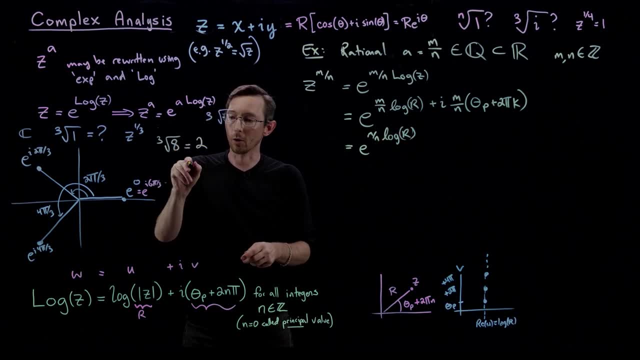 of the magnitude of eight. So that would be two or two times e to the i two pi thirds, or two e to the i four pi thirds. So this is just the magnitude part. If I didn't, you know, if I had something that was non-trivial magnitude. 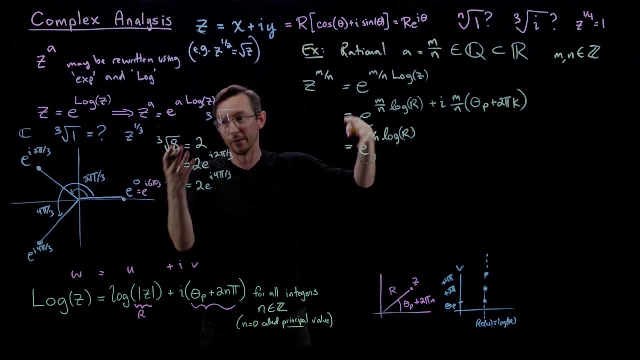 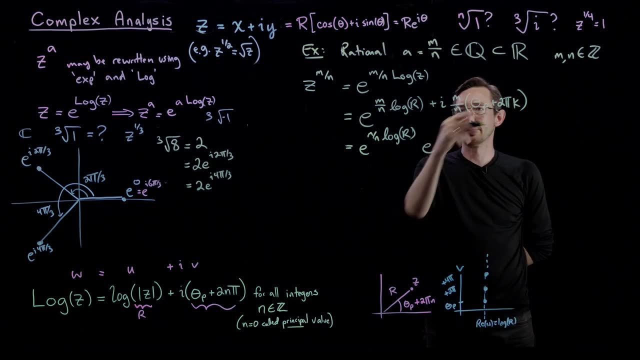 like length eight instead of length one, I'd have to take the third root of that length as well. Okay, so there's that times e to the. i I'm going to break this up. I'm going to say this is e to the. 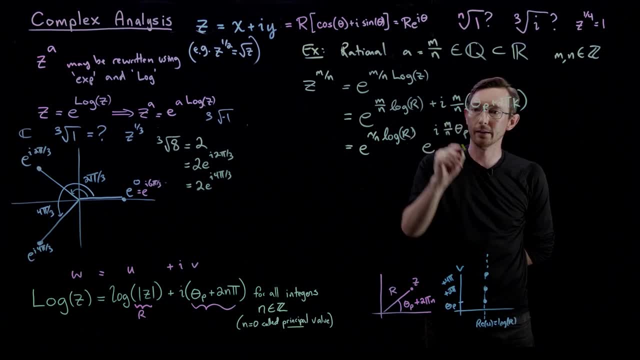 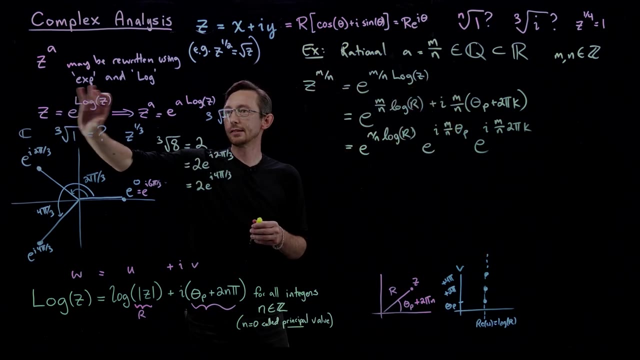 i m over n theta p times e to the i m over n two pi k. okay, That's all I've done is I've just taken z to the m over n, I've used this formula for it and I plugged in the complex logarithm. 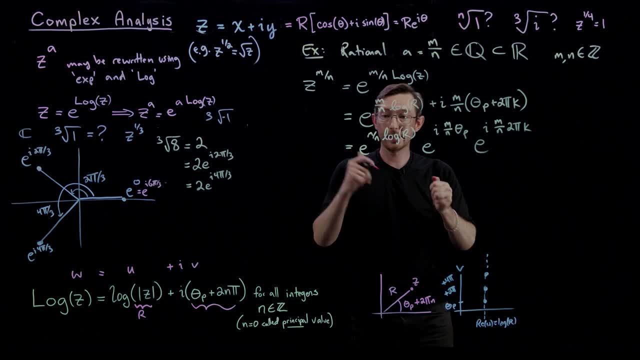 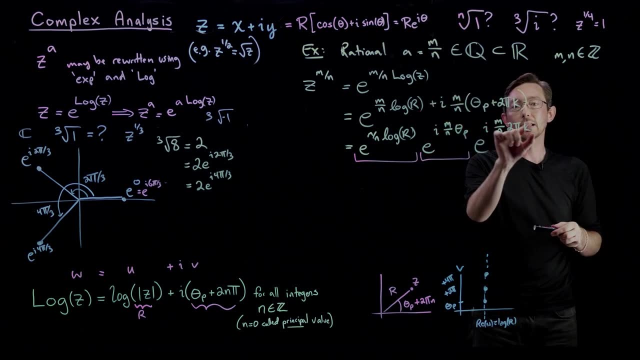 and I've gotten these. Now, this term is single-valued, and this term is single-valued. this term is true for any integer: k, k1,, k2, k3, k0, and so forth. And so now what we're trying to do. 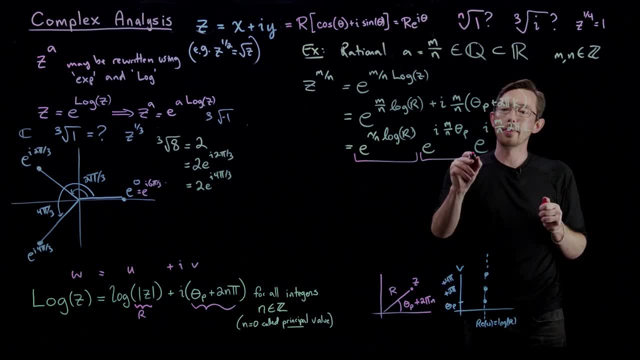 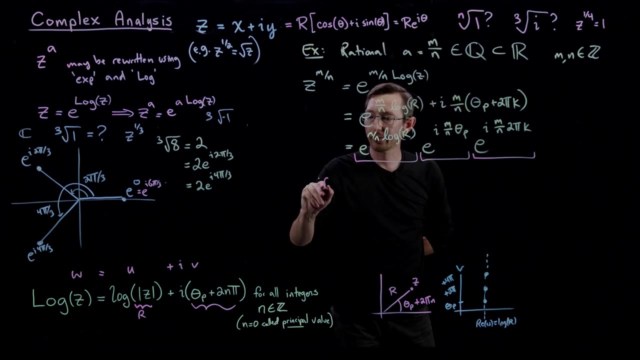 is we're trying to find. you know, there are only so many unique values of this quantity before it starts repeating on itself, which is what we saw here. So, for example, if you know, if m over n equals one-third, 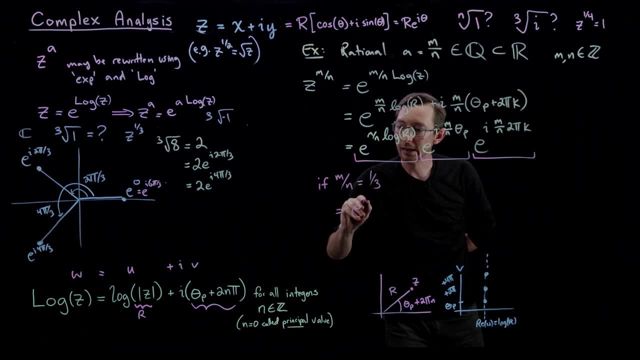 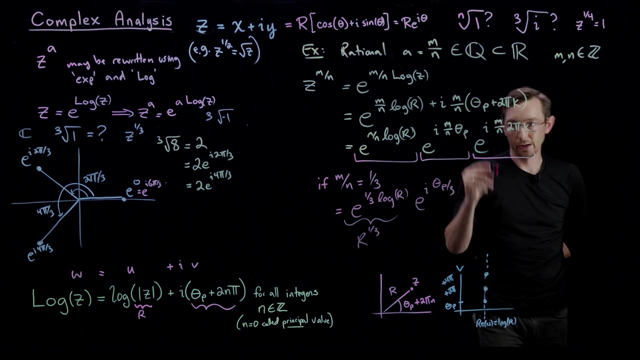 then this would be equal to e to the one-third log of r, which is the same as r to the one-third. This would be e to the i theta, p over third over three, and this would be e to the i two pi k. 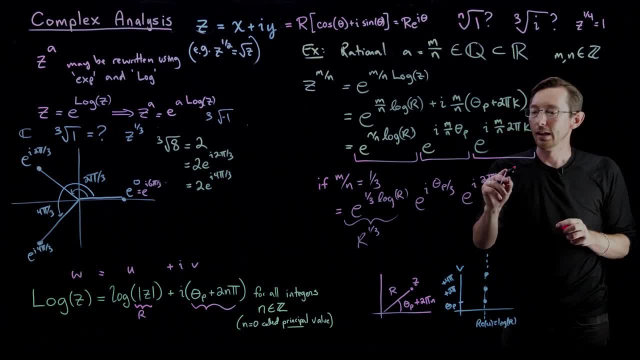 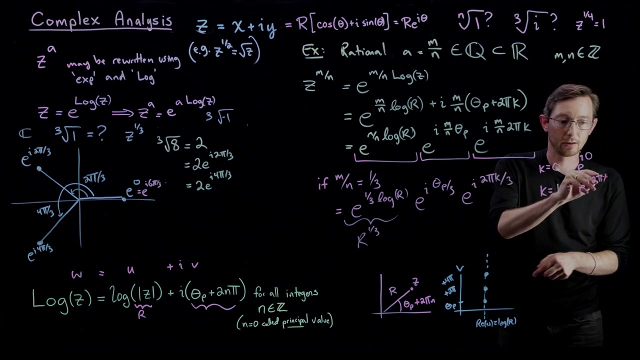 over three, And what I claim is that there are three unique values of k, where this, this is unique. So let's try: k equals zero, then this is e to the i zero, That's fine, k equals one. that would be e to the i two pi thirds. That's one of my principal. 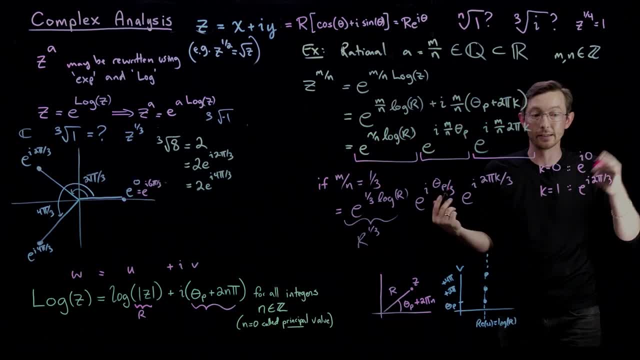 cubed roots of one. That's fine. This is different than e to the zero, That's a. these are different numbers. k equals two would be e to the i four. pi over three. Again, that is a different number than either of these two. This is an actual different. 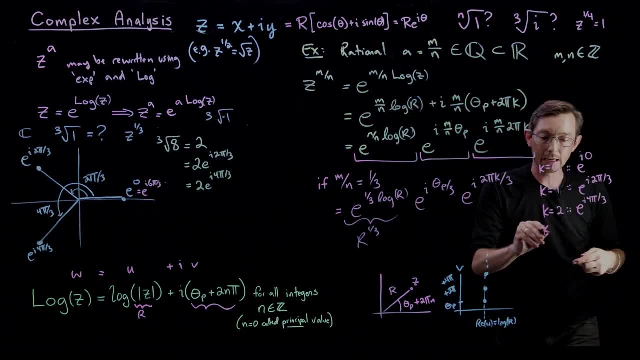 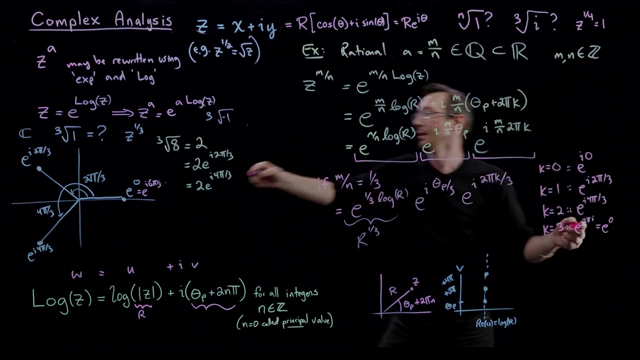 complex number than these guys. okay, But when I go to k equals three, I come back to where I started. If k equals three, here I have e to the i, six pi thirds, which is e to the. you know, two pi i, which is the same as e to the zero. e to the two pi is e to the zero. This is. 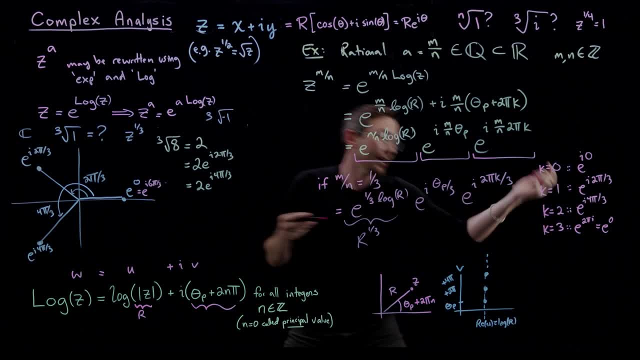 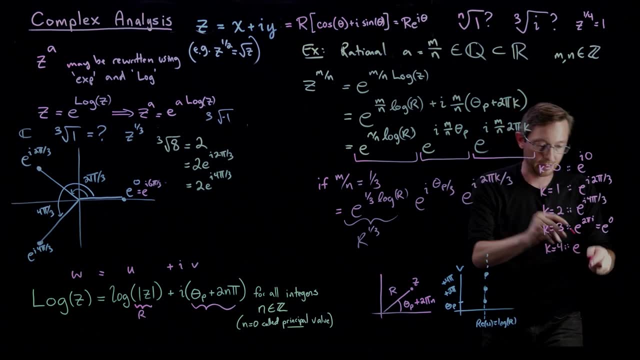 this is the same as k equals zero, And I'll just I'll show you. you know, k equals four is e to the goodness gracious eight pi thirds. you know, i eight pi thirds, which again is the same as e to the i two pi. 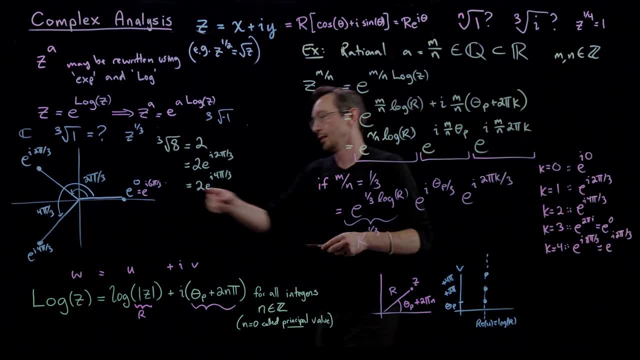 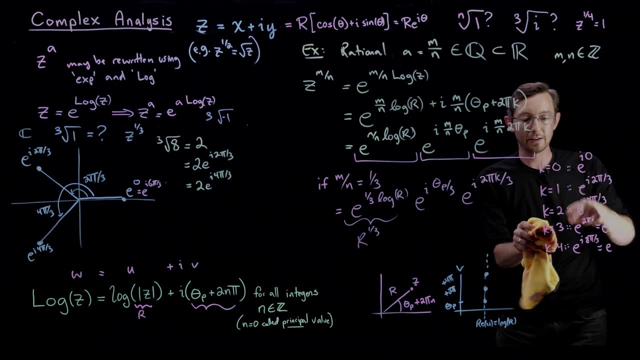 thirds. These are the same number. It's just. you know you, just you've gone all the way around, And so what this means is that there are only three unique values of k, where these numbers are actually different. k equals zero, k equals one. 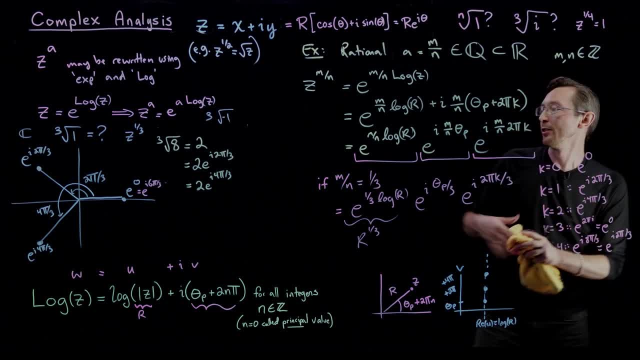 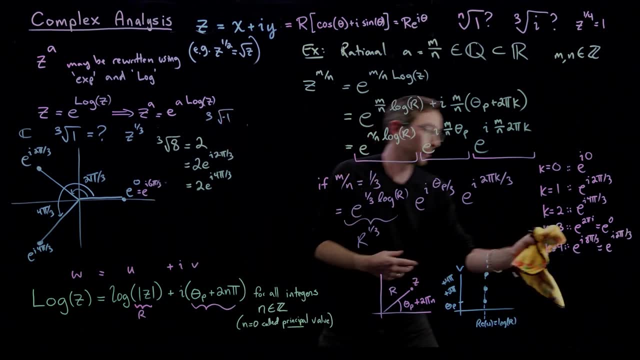 and k equals two, And for all of the other k's you've essentially just gone around and re-found this number or re-found this number, or re-found this number, you know, and over and over again. So so I think that that's really really interesting. That kind of shows why. 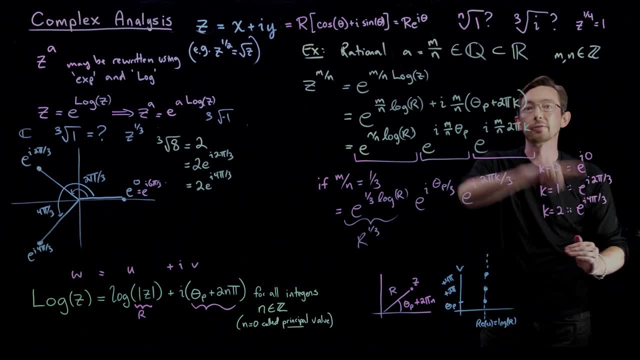 And if this was one fourth, there will be four unique numbers before you get back to where you started. If this was one fifth, there would be five unique numbers before you get back to where you started, And that's why there are three unique cube roots of. 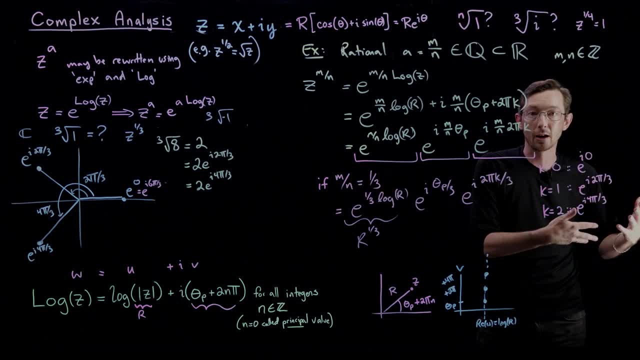 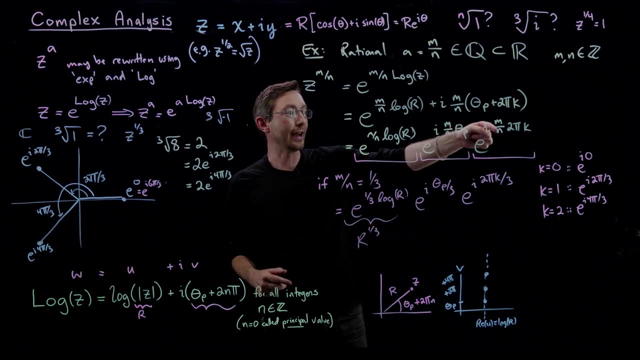 uh, complex number. There are four unique fourth roots of a complex number, and so on and so forth. Okay, It's, it's literally, because this complex logarithm, when you divide, when you, when you multiply it by this rational number, there are exactly n unique values of k that give you 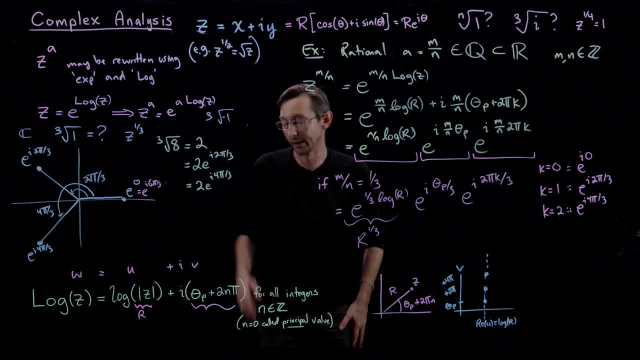 different numbers for this quantity here, after which it starts recycling back on itself. Okay, I think that's super duper useful. Uh, and this means I can take the fourth root of i. I can take the ninth root of one plus i. I can take any complex number I like. 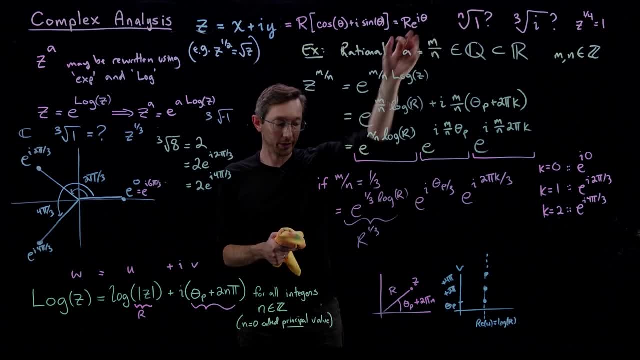 and if I write it in polar form with a principal angle, and I use this formula for the logarithm, I can find every single nth root of this complex number. I can take z to the one nth or the two nth or three nth or whatever, and I can find all n unique roots of that uh, of that number. 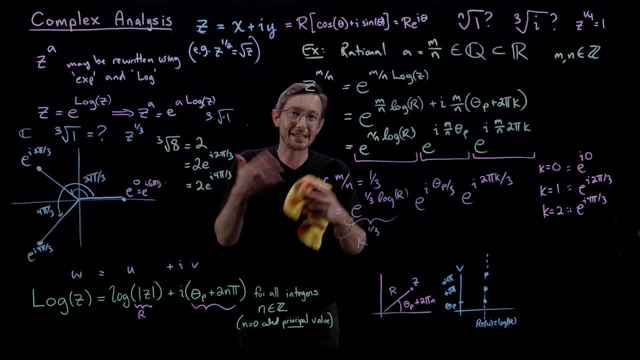 Sometimes these are called um, there's a uh, a saying in complex numbers called the roots of unity, the third root of one, the fourth root of one, the fifth root of one, because they form these kind of canonical uh pictures that you. 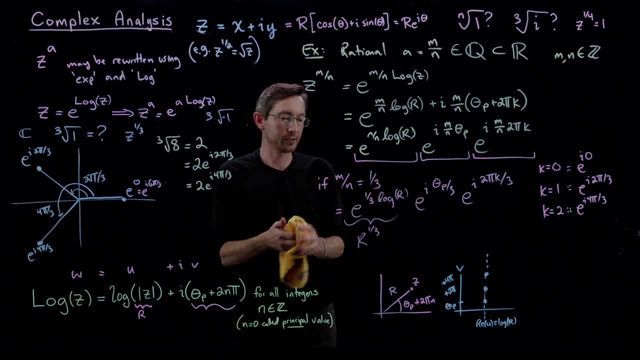 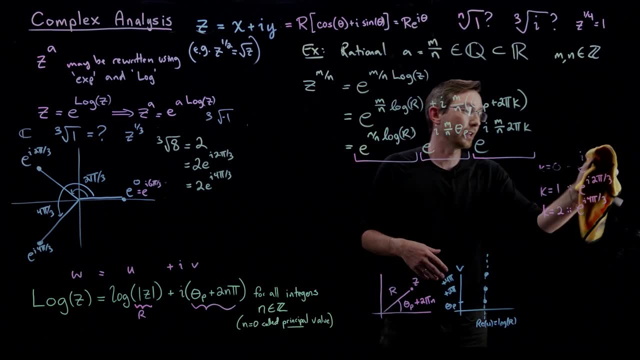 can use to compute other roots of other numbers. Good, Um, this actually begs the question. There's some really weird stuff that happens if you take uh z to the uh, a rational number. If I take, you know if I take z. 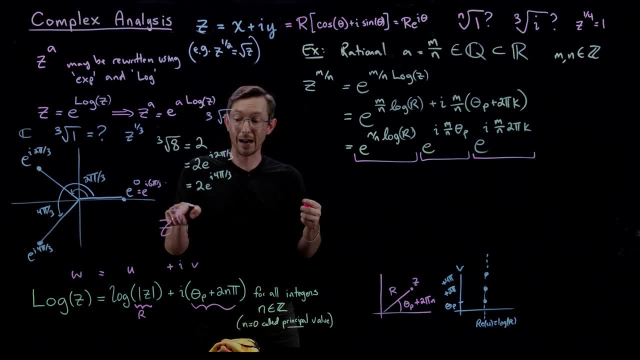 to the, the pi-th power. this is an irrational number. There is not, there is not uh, an integer m and n that I can write, uh, pi in terms of, And so if I take, like you know, negative one to the, 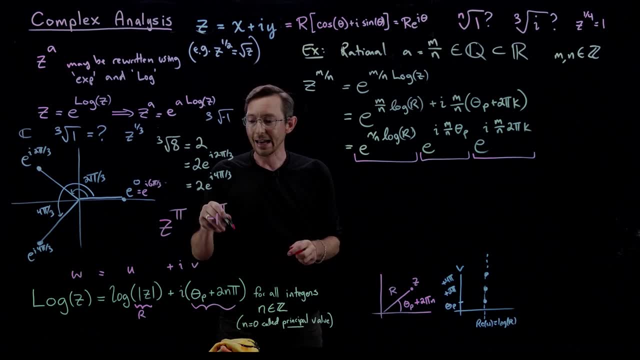 pi-th power. there are infinitely many. this is super weird. there are infinitely many values of negative one to the pi-th power because for every single k, you know, for every single n here, for every single k here, if I, if I plug in a pi here, there are infinitely many values of this. uh, and. 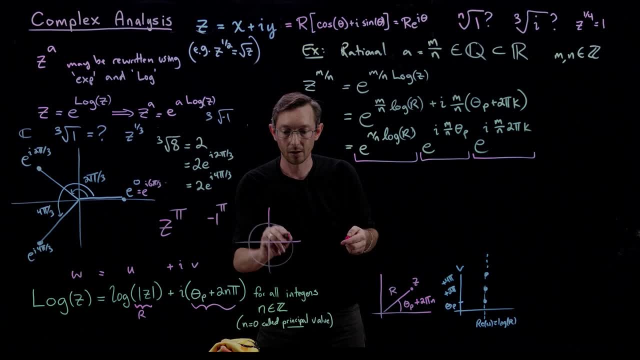 in fact, I would say that any number here on the unit circle is a solution of negative one to the pi-th power. That's a very weird and strange outcome of the fact that log of z is infinite valued and pi is irrational. It's a weird thing, but it's true. Um good, What else do I want to? 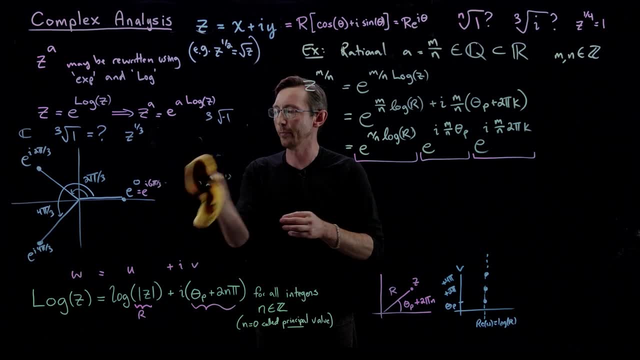 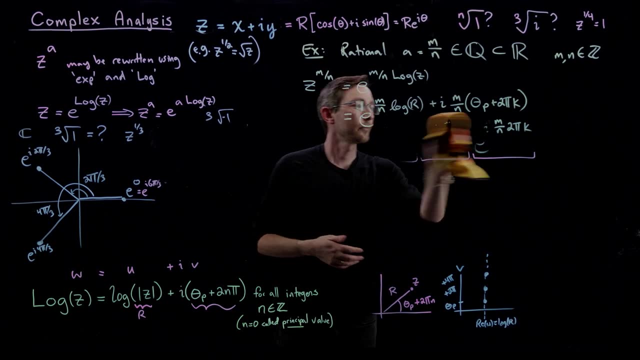 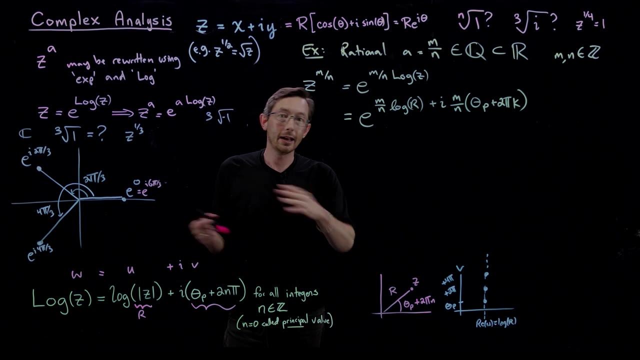 say: Uh, maybe I'll just do a couple more examples, because I think this is really helpful. Um, let's see, let's see, let's see. Okay, I'm just going to erase this. Looks actually like this formula better. Uh, let's do the fourth root of i. 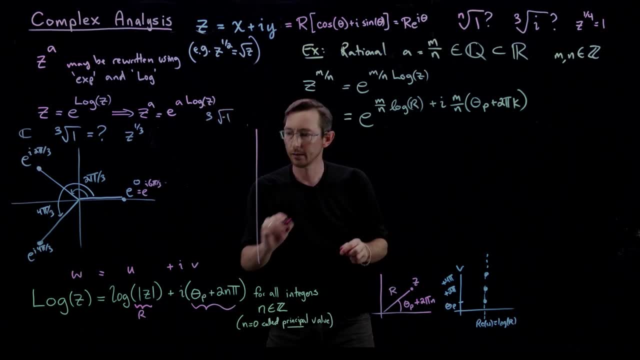 and then we'll call it quits. Okay, so if I take uh, sorry for the squeaky pen, So let's say uh, I have uh. or let's take, you know, the fourth root of 16i, because I want to show you what happens if you have a non. you know, if it's not length one. 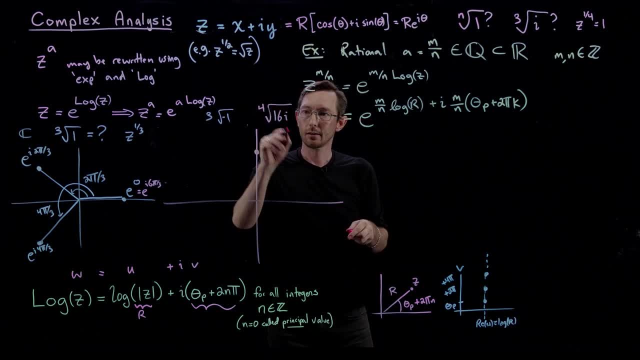 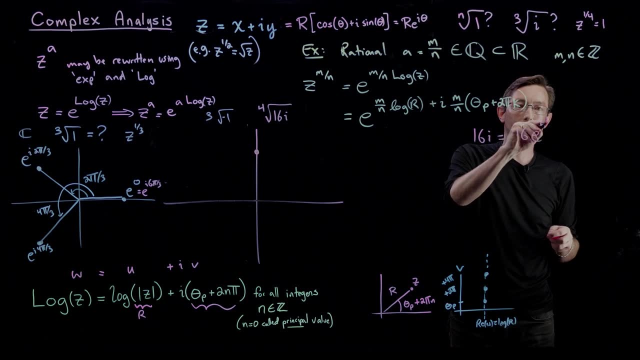 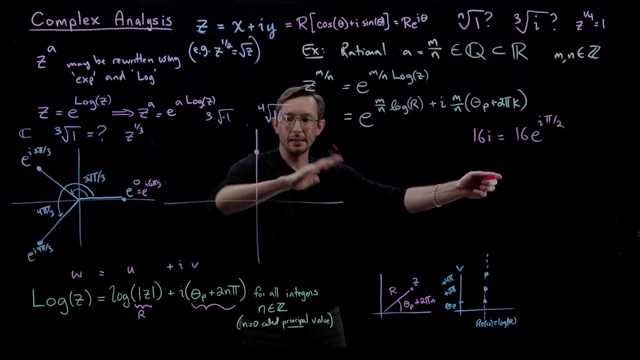 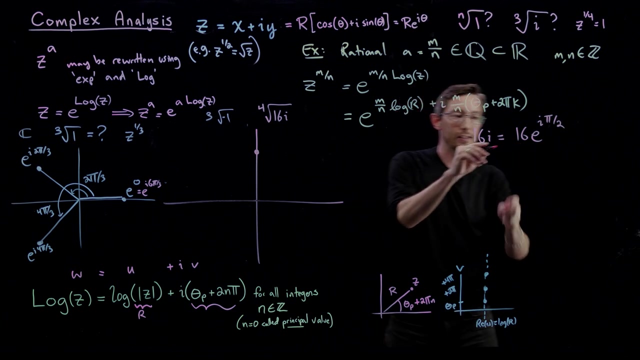 So in this case, um well, let's write: 16i is equal to 16, e to the i pi-halves. Okay, so the number i is just e to the i pi-halves, because it's in the pi-halves angle and 16i has a radius of 16i. 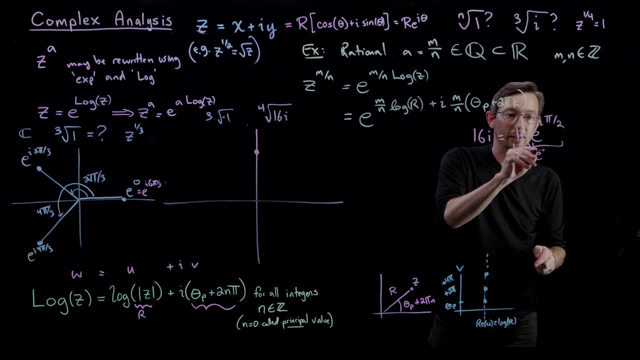 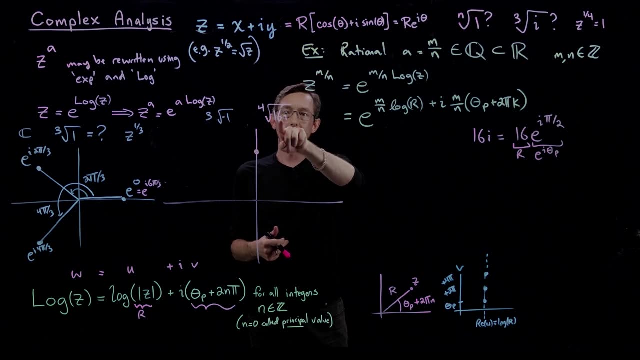 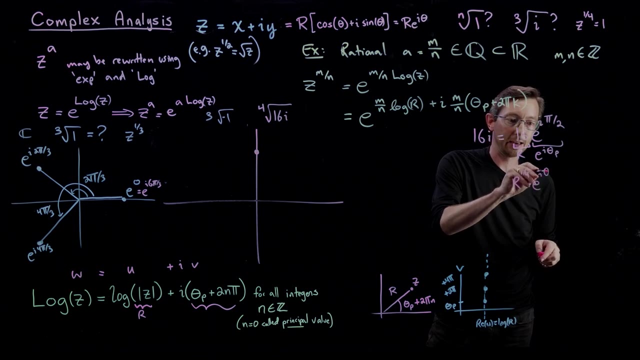 So this is the radius and this is, you know, e to the i, theta principle. Theta principle is pi-halves, And so if I want to take the fourth root of 16 i, I basically take, you know, r to the one-fourth and then e to the i. 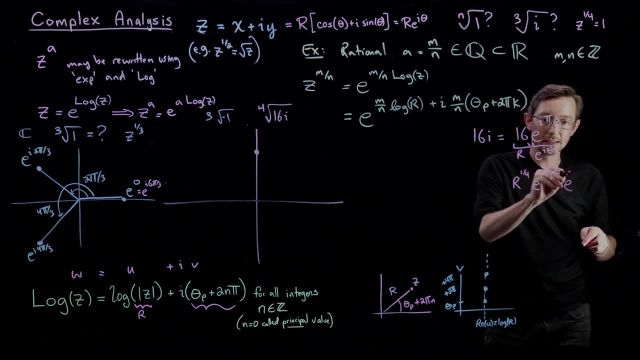 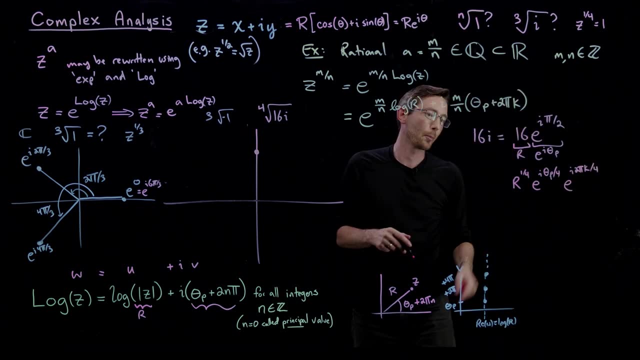 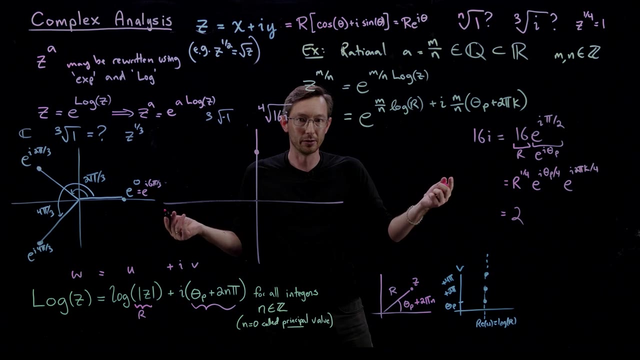 theta p to the one-fourth times, e to the i, 2, pi, k, fourths for all integer k, until it recycles on itself. Okay so. So the radius to the 1 4th equals 2.. I chose 16 because its 4th root is 2.. 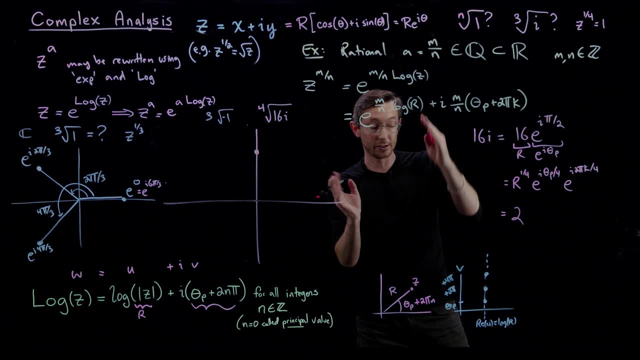 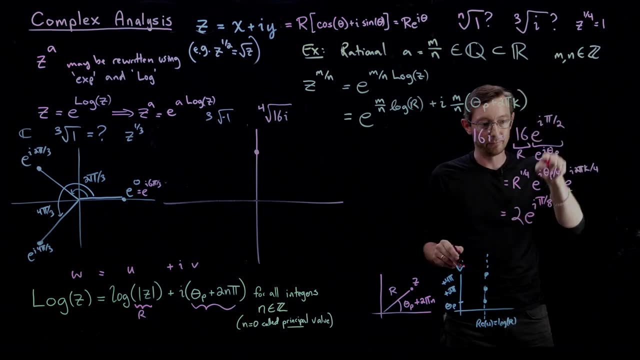 So the magnitude of all of these 4th roots, they're going to have radius 2.. This is e to the i, pi 8ths. okay, because that's what the principal angle divided by 8 is, And this is really easy to understand. 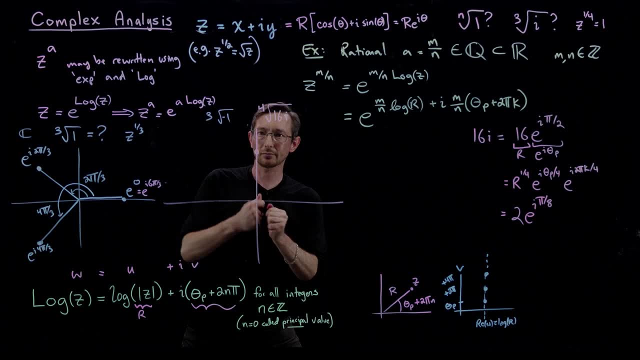 If I took this, you know this is, let's say, let's say this is 16i, then the first principal, 4th root of this is going to have- I'm going to divide this into four pieces, So it's going to have length 2, e to the i pi 8ths. 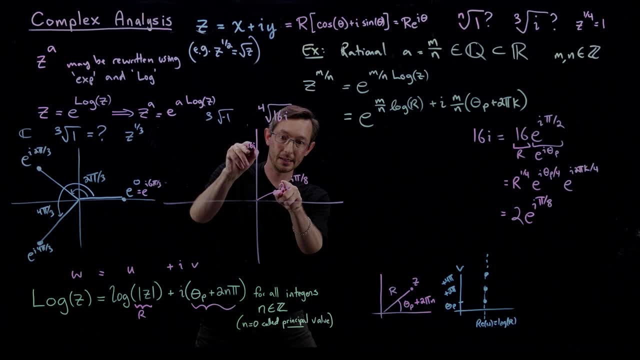 Because if I took this to the 4th power, I would get: 2 to the 4th is 16, and e to the pi 8ths to the 4th power is e to the i pi halves, which is this: 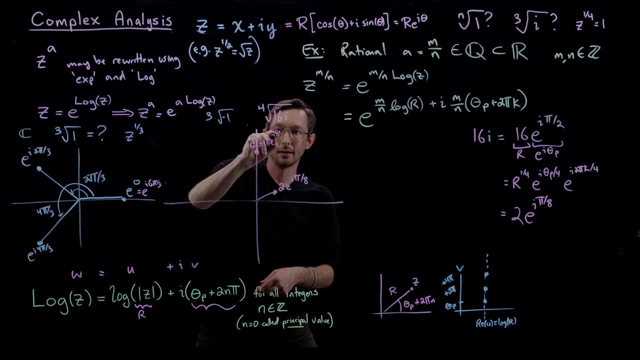 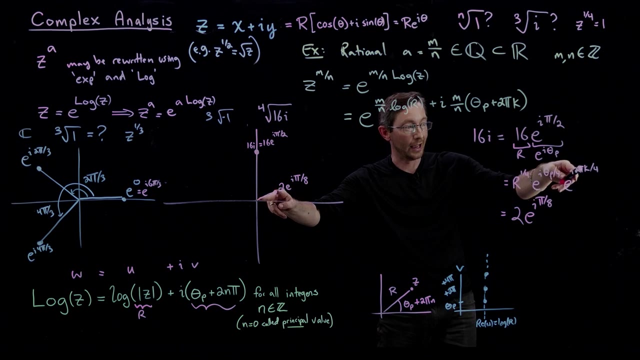 This is, you know, 16 e to the i pi halves. So this is my first principal 4th root of 16i. But now I also have this: plus 2 pi 4ths, plus 4 pi 4ths, plus 6 pi 4ths. 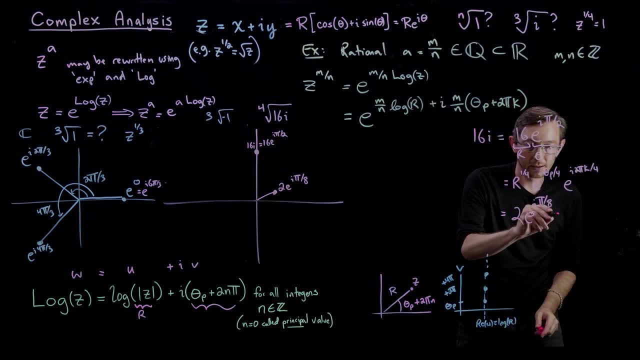 and so on and so forth. So e to the i and I'm just going to say, you know, 2 pi 4ths is pi halves, pi halves k, And I'm going to choose k until this thing recycles on itself. 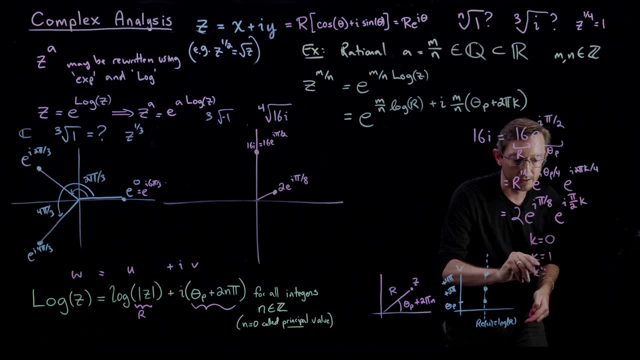 So k equals 0, k equals 1, k equals 3.. Can't count, This has been a long day. k equals 3 and k equals 4.. So at k equals 0, I just have 2 e to the i pi 8ths. 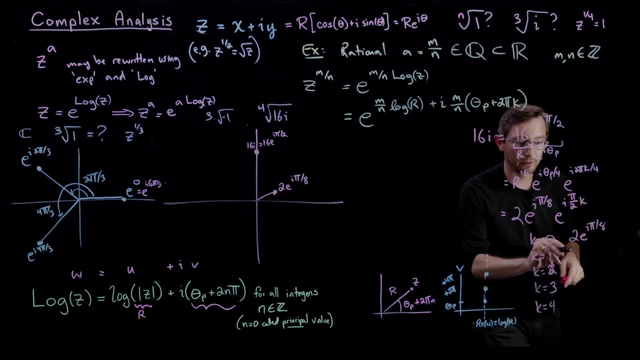 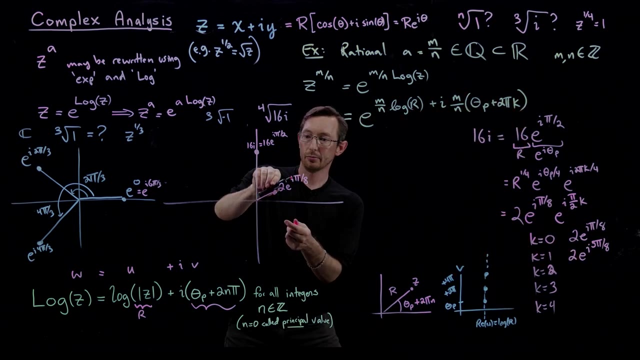 That's the solution here. For k equals 1, I have 2 e to the i pi 8ths plus i pi halves. So that's i 5 pi 8ths For k equals 2, and 5 pi 8ths is just this plus pi halves. 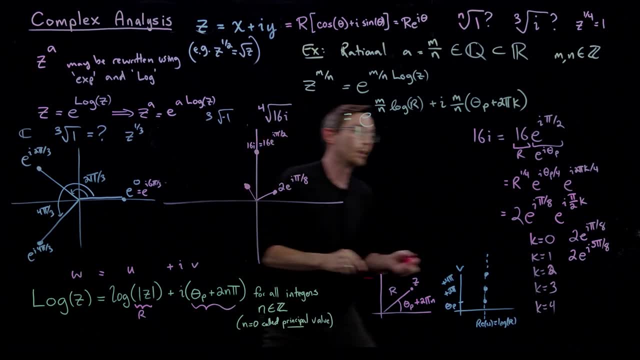 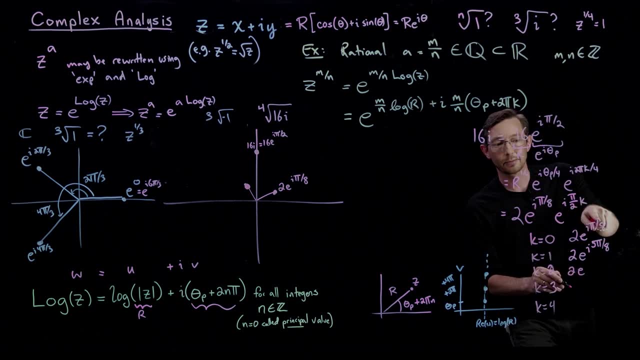 which is a little hard for me to draw, but it's something like that: If I have k equals 2, then this is 2. e to the i pi 8ths plus pi, which is goodness That's going to be i 9 pi 8ths. 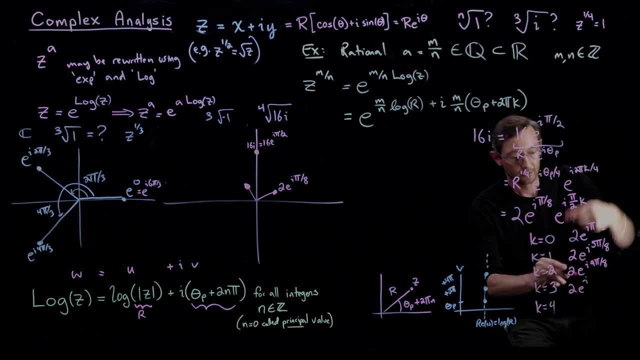 I'll do. k equals 3 is 2 e to the. i probably 13 pi 8ths. And by the time I get to k equals 4, I'm going to get 2 e to the. i add 4 again. I'm going to get 17 pi 8ths. 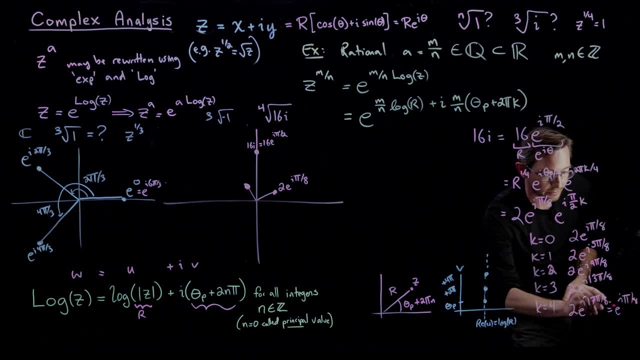 which equals e to the, i pi 8ths. So by the time I get to k to the 4, to the 4th k and the 5th and the 6th and the 7th and the 8th here, 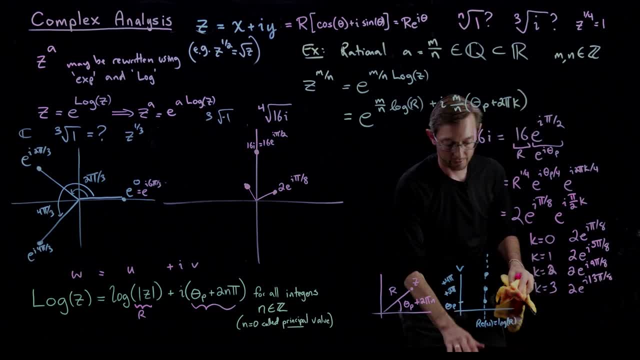 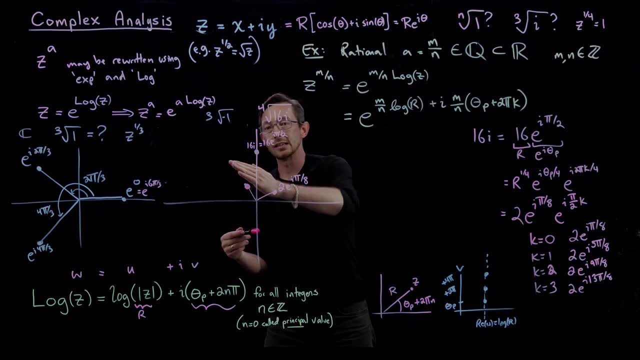 I essentially have rediscovered the same numbers that I was using originally. So for k equals 0, that's this one. For k equals 1, it's this one. k equals 2, each of these, I'm just adding pi halves. 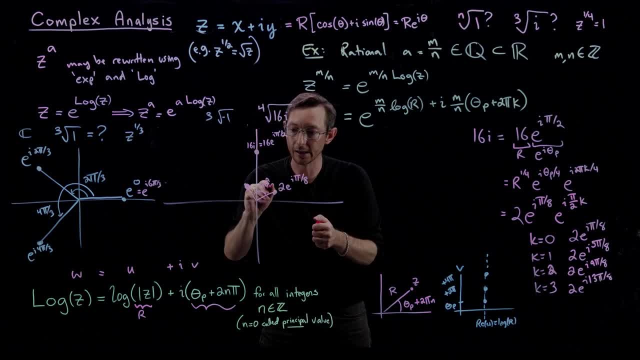 I'm just rotating by 90 degrees. This is just, you know, 90 degrees or pi halves. So the next one is going to be here, and the last one is going to be here, And what's really cool is that all of these nth roots. 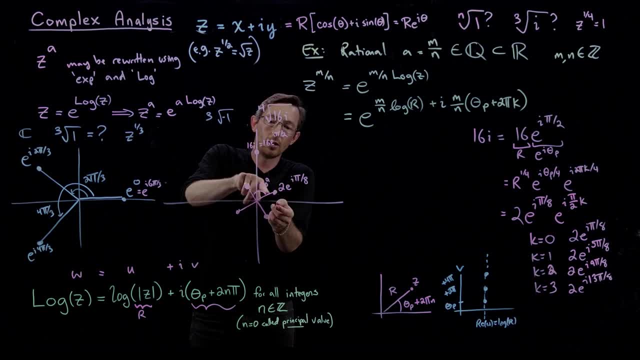 of any nth of any number kind of form, this star pattern, where they all are equal, distant to each other, dividing 360 degrees. So these, you know, were each 120 degrees separate, or 2 pi 3rds separate, 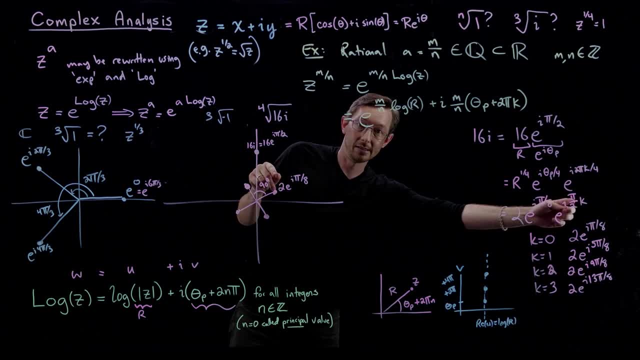 Each of these are 90 degrees or pi halves separate And at some point there are only 4 unique 4th roots of this number, because after the 4th unique one, the next one, I'm basically back where I started. 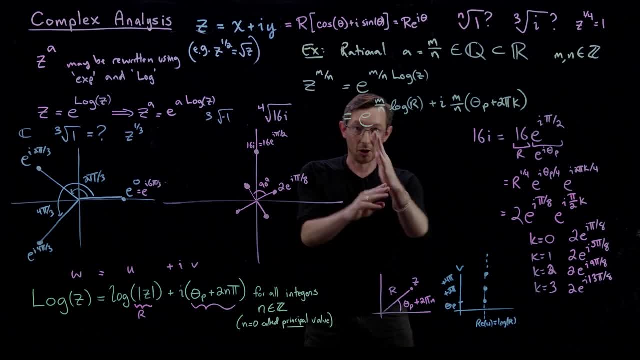 And if this was the case, if this was the 5th, you know, nth, root, I would get a star pattern with 5,, you know, like a pentagon, I would get things equal, spaced 5 ways. If I took the 6th root, I would get things equal, spaced 6 ways. 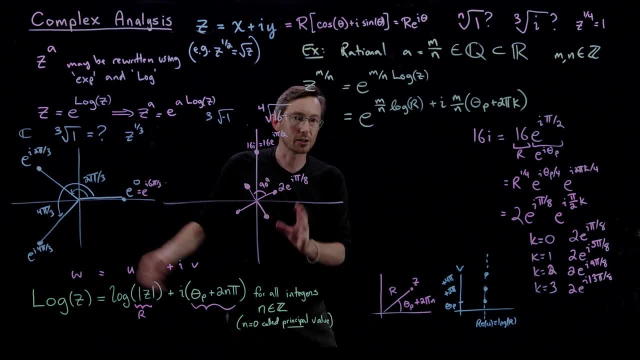 and so on and so forth. So it's really cool There's this kind of geometric picture. but this is all related to the fact that the complex logarithm is infinite valued, And so you can use that when you're computing z to a fractional power.